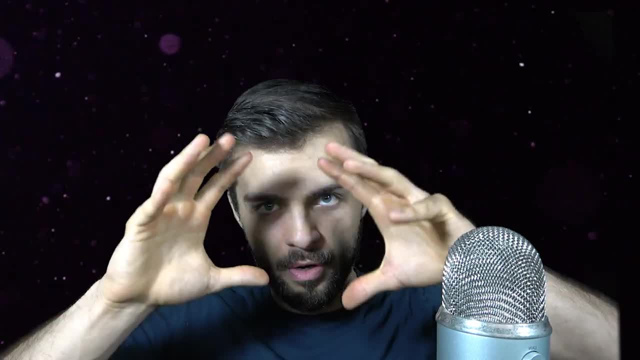 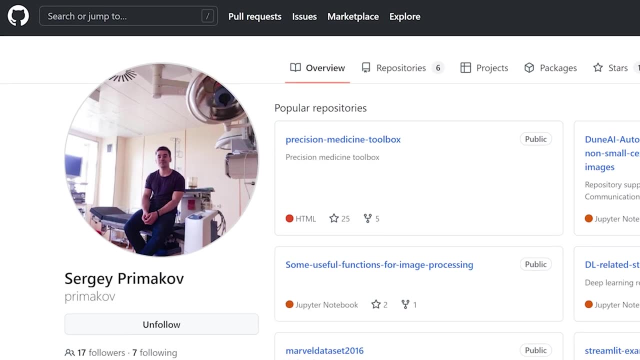 So the other day I was reading a paper with research that I was doing which involved segmenting the lungs from a CT scan, and I found this github profile here from a guy named Sergey Primakov. So shout out to whoever you are from Maastricht University. and he had. 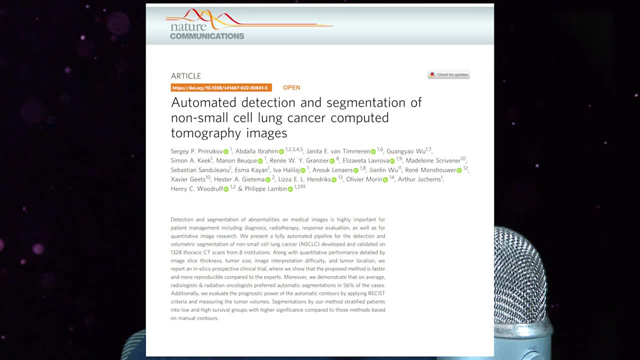 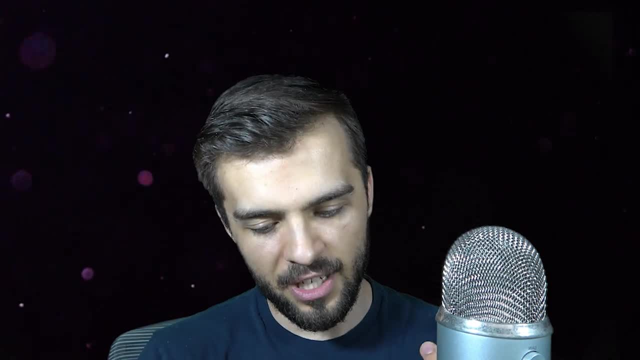 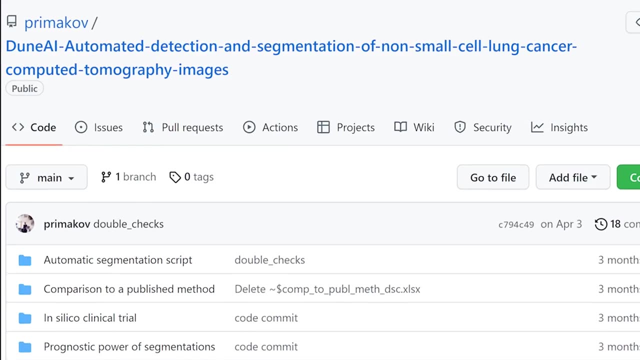 written a paper in Nature Communications. By the way, Nature Communications is a very highly reputable journal- and I noticed in the article that he actually provided the code from his project where he segmented the lungs publicly and it's actually right here and you can take a look at it and this is state-of-the-art stuff and he's using all the modern python libraries. 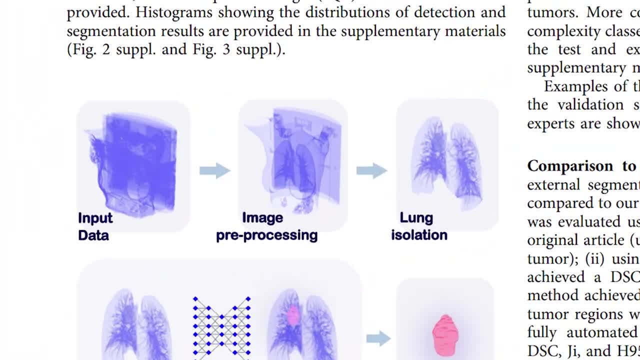 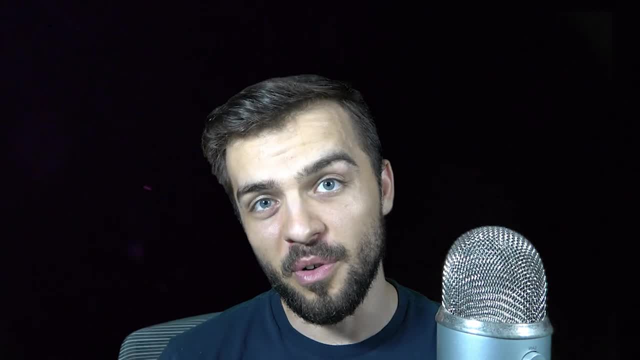 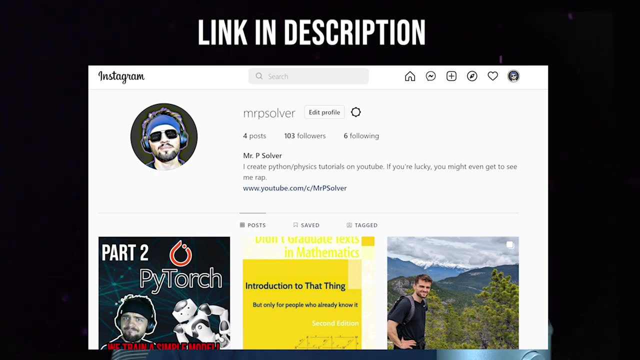 to take, basically, a 3D CT scan and just return a mask of the lungs, and so that's what we're going to look at in this video. If you enjoy this video, please remember to subscribe. as always, join the discord server as well. and finally, I just started an Instagram account for this channel as well, so 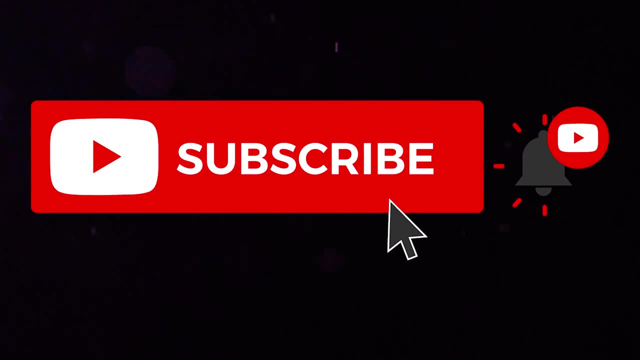 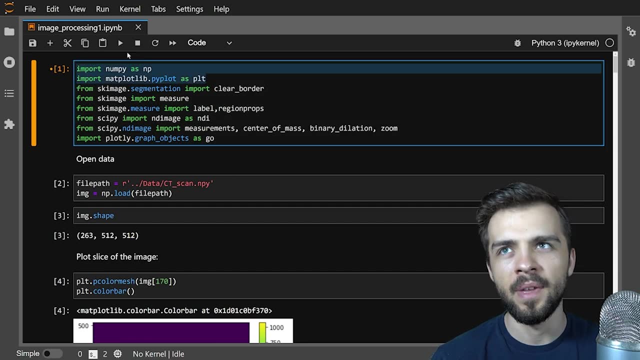 check that out. So the packages today are kind of important. we have numpy and matplotlib as normal, but the main image processing stuff that is state-of-the-art in python that we'll be using is. scikit-image is a beautiful image processing package. it's got a little bit of machine learning stuff: scikit-learn. 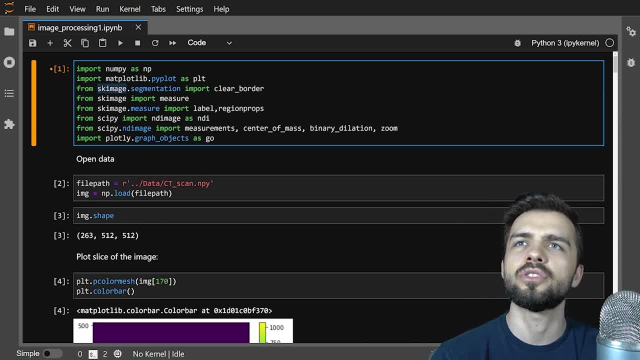 is the machine learning library associated with it, and then also scipy. we have some stuff from the nd-image library which is going to allow us to do make measurements of the image compute center, of mass, of various regions and some other functions that we'll get into in this video. so the first thing is we're 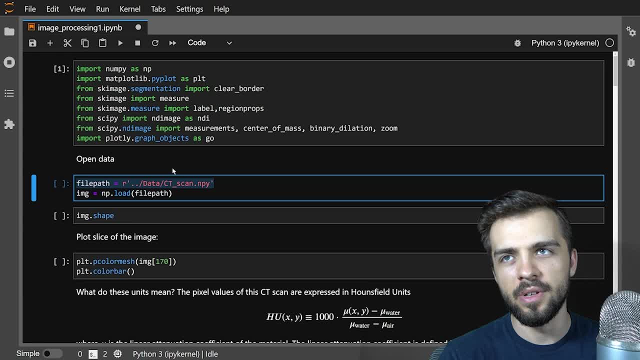 going to do is we're going to open our data. I've put this data in the git repository so you should be able to access it. it's just one directory back in the data repository. it's a ct scan and we'll look at it, and so here I just load it using numpy, and the first thing to do- and this is something I 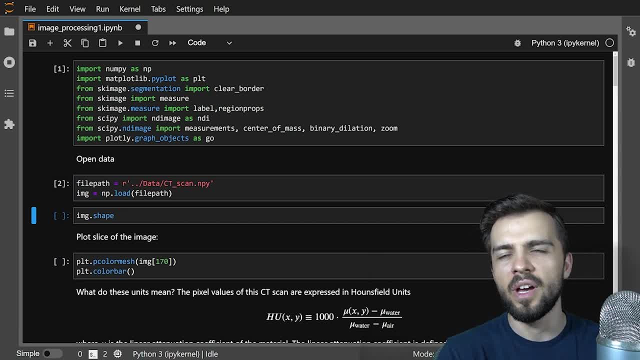 do always when I'm doing machine learning with images or any sort of array that I open. the first step you should always get used to is: you're going to want to make sure that you've got a lot of data in the data repository and you're going to want to make sure that you've got a lot of data. 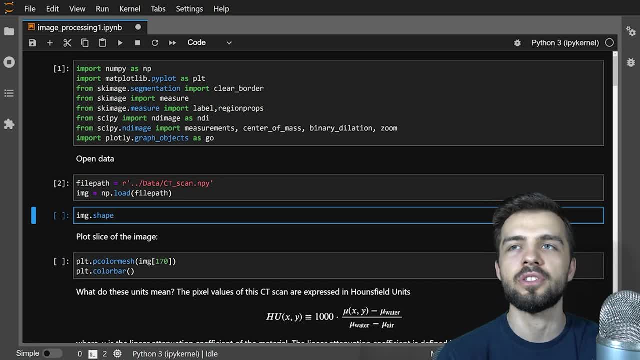 in the data repository- and you're going to want to make sure that you've got a lot of data to- is looking at the shape of the image, because this will tell you about what you just opened. so I have no idea what to expect here. well, actually I do, but you know, you might not have. 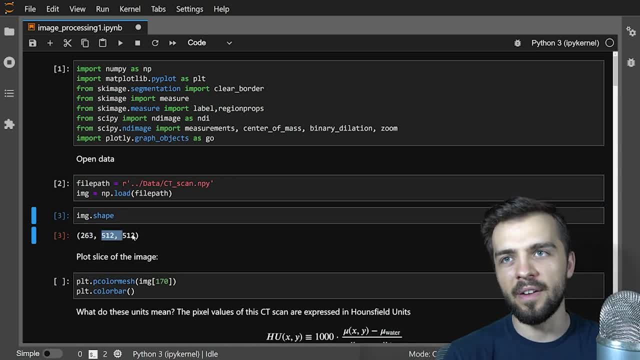 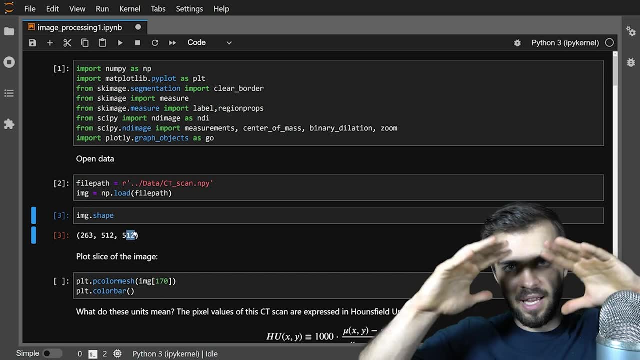 any idea what to expect. and you see, the shape is 263 by 512 by 512, and the shape is the shape of the image, and so what you have here is not a 2d image, but a three-dimensional image, and so what it is is that 263 is along the height of the person. so from 0 to 263 and then the 512 by 512. 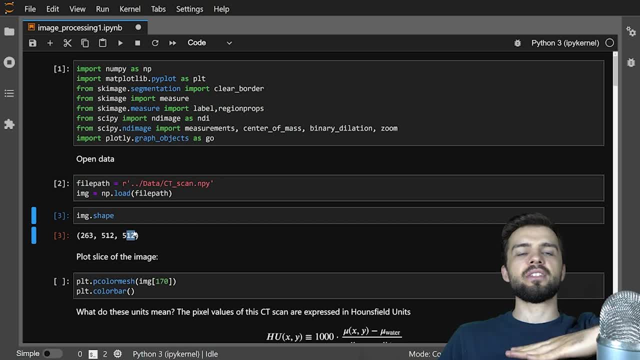 is like you're taking slices of a person, sort of like this. it's called an axial slice, and so you have a 512 by 512 image and you have 263 of them and they're sort of like a sliced ham of a person. so we'll look at that, and so what it means is we're looking at a 3d image and what we want to. 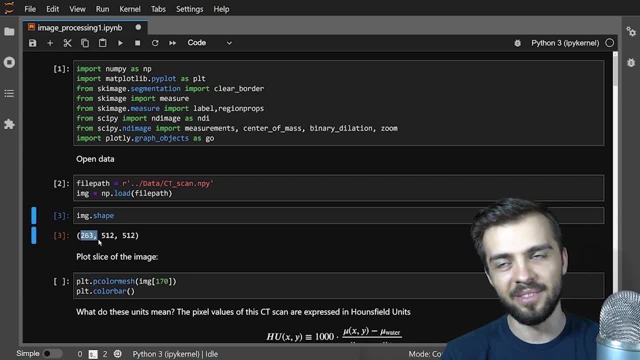 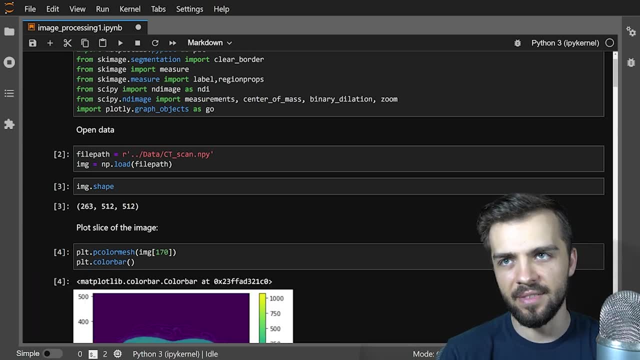 do is: we want to process all of these slices and I'll let you know what our goal is pretty soon. so let's look at a slice of the image. here I'm going to take the 170th slice of the CT image and you can see that our image is here. 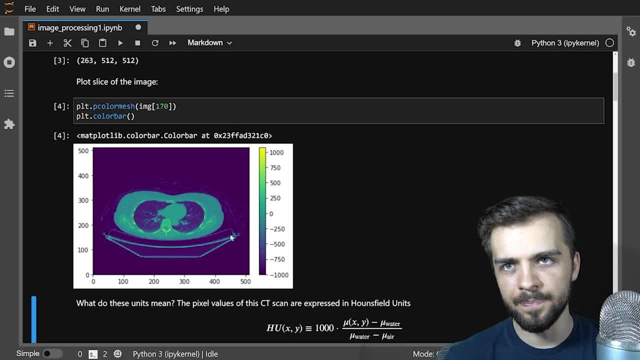 and what you're looking at here is, well, at the bottom you have the table and it looks like this, and so the table is sort of whatever 500 is, and then it's sort of an air gap in the center of the table and then you have like a slice of a person, sort of directly like this: it's like you cut. 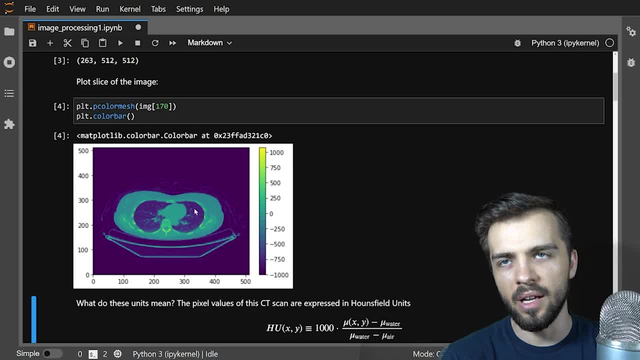 someone up like a ham and you're looking in here and what you have is the two lungs and then you have all the tissue on the outside and you have this sort of arbitrary scale and you might not know quite what it is, and we'll get into that. so the first thing to do, we're looking at a new type. of data. we should probably understand what we're looking at, and we're going to look at what we're 研究的是我們正在明白為何 우리가落得所在的所為. 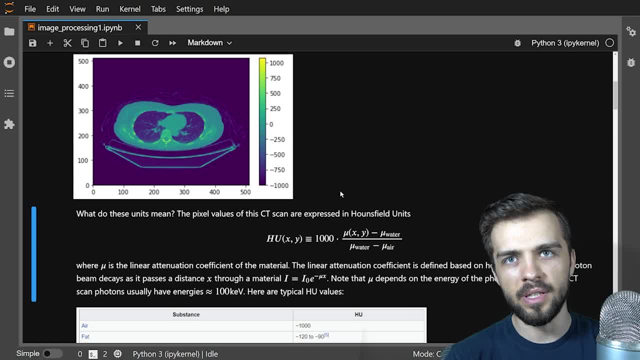 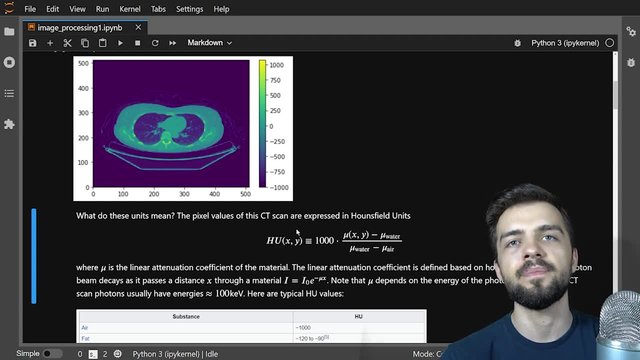 address scale means, and so the units correspond to hounds field units and a hound's field unit um at every point x, y. so each pixel value has a hounds field unit, uh quality. so I give an x, y, you'll tell me how many Jean Suderle units it is, and that's the uh value given by the color bar. 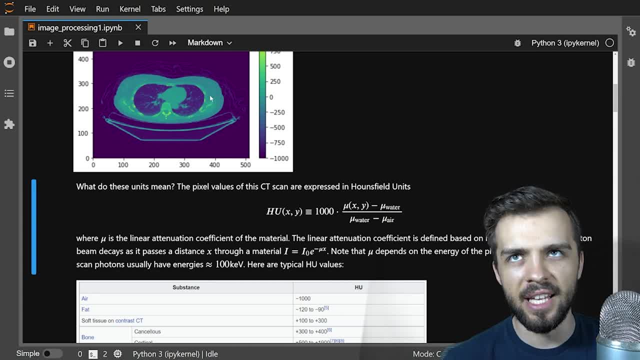 here it's equal to a thousand times whatever the attenuation coefficient is at that location in space, minus the attenuation coefficient of water divided by the difference between the attenuation coefficient of water and air. and so you might think: well, why are you using this scale? this seems a little bit bizarre. and there's also the linear attenuation coefficient which is defined. 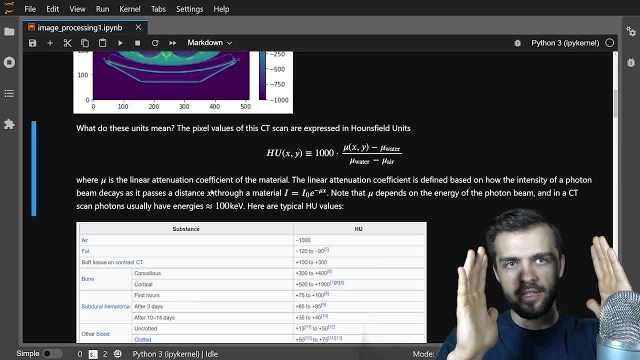 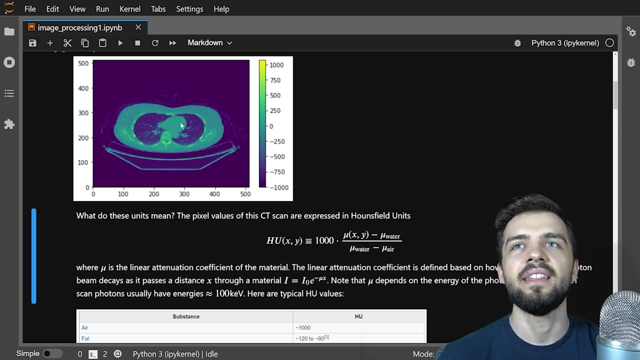 such that if i have a beam of intensity i naught coming into a material of length x, the intensity coming out is going to be i naught e to the negative mu x. so it's how many photons get attenuated in the matter. so the higher attenuating this is, the higher the probability that an x-ray 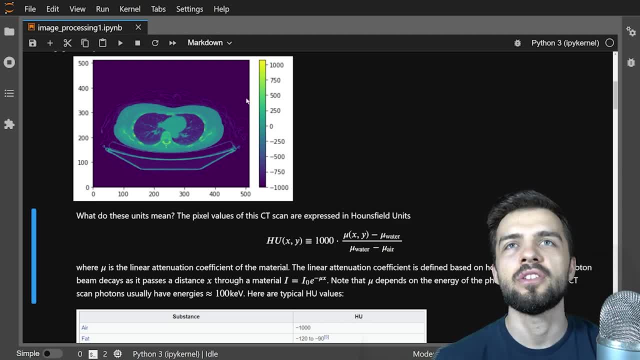 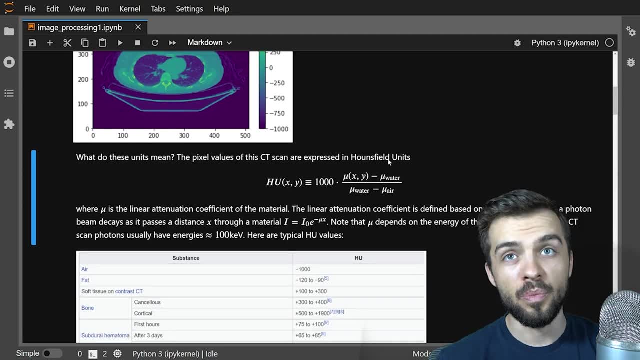 shining through your body gets absorbed by your body. so these higher regions here correspond to higher probability of attenuation and it's sort of scaled like this, and so the reason they define it like this is it gives a really nice scale for differentiating between different types of tissue. 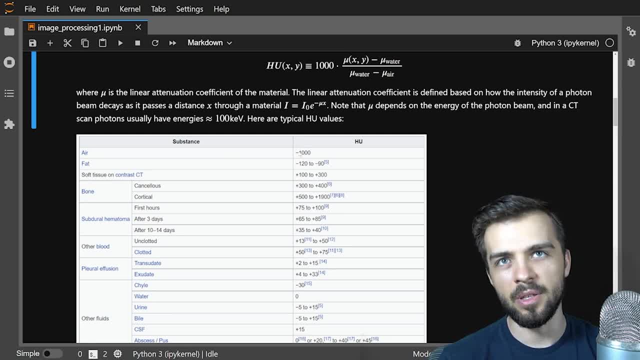 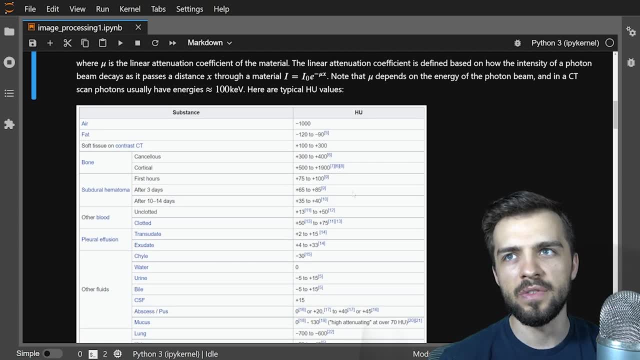 so here i have, for example, air is minus 1000, that's just something you remember. a fat is minus 120 to minus 90, and then you got soft tissue- 100 to 300. you have all these different values for bone, blood and sort of all these different values for air, and then you have 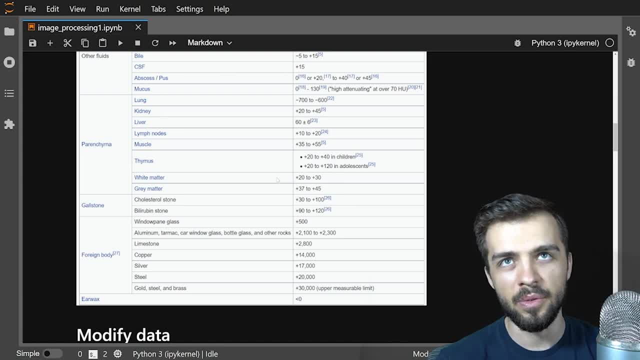 all these different values for blood and sort of all these different values for air, and then you have this stuff here and you can determine exactly how many houndsfield units something is. so looking at this image, you can look at a particular color and it tells you something about what material. 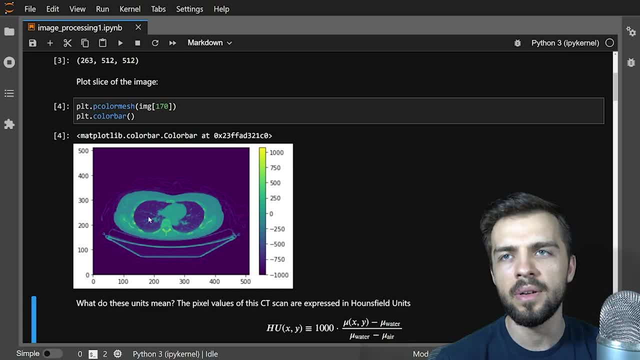 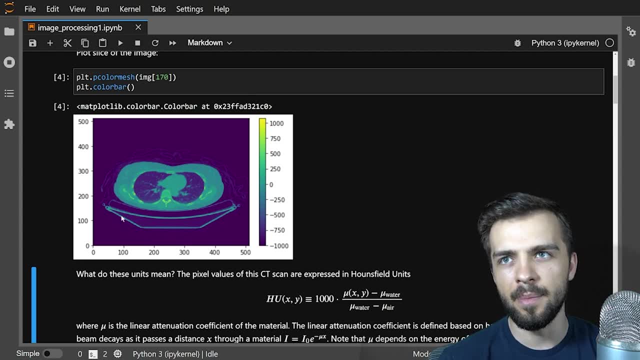 the actual point in the image is made up of. so maybe there's bone here in the lungs. you can see it's close to minus 1000 because the lungs are mostly air. the same thing on the outside and the table is pretty attenuating. so it must be made of some sort of metal and then there's sort of an air. 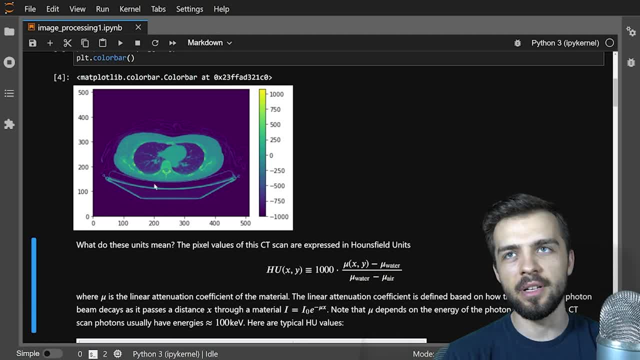 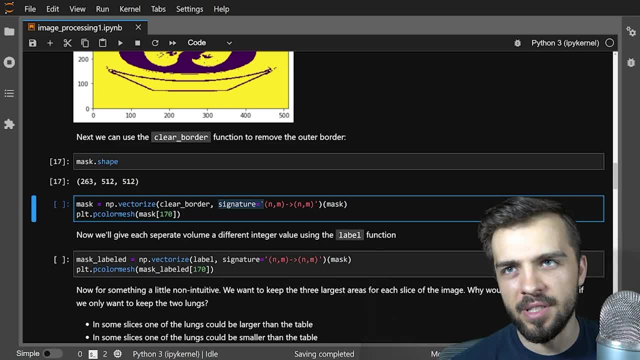 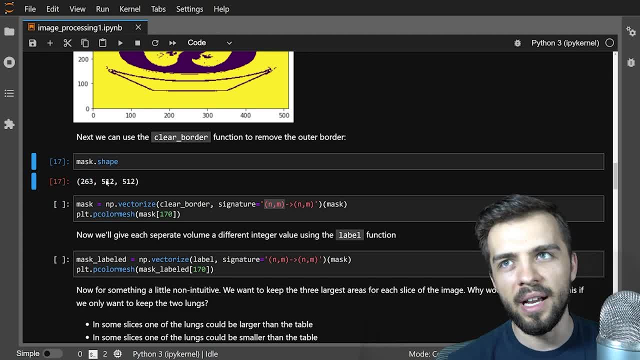 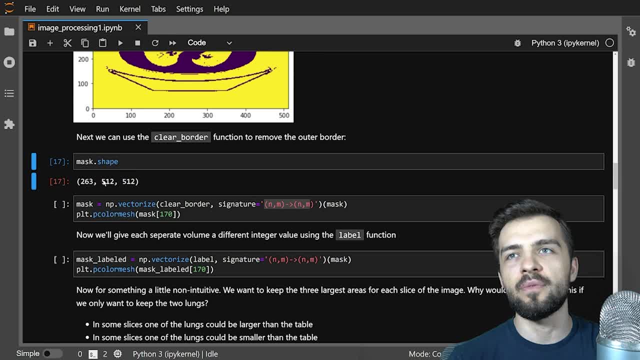 every element of the array. You don't want that. You want it on every 512 by 512 slice of the array And for that, that's why you have to give this signature of saying we're giving it a 2D array and it's returning a 2D array in this clear border function. So I'm vectorizing clear border. 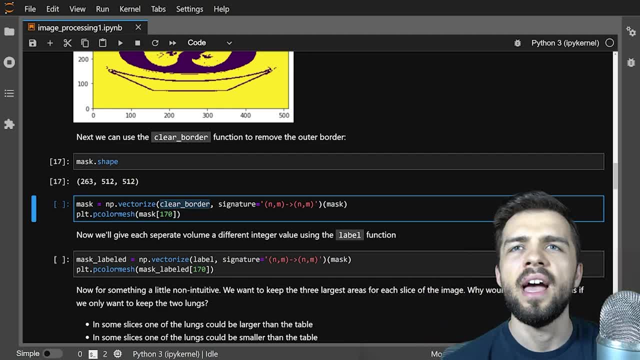 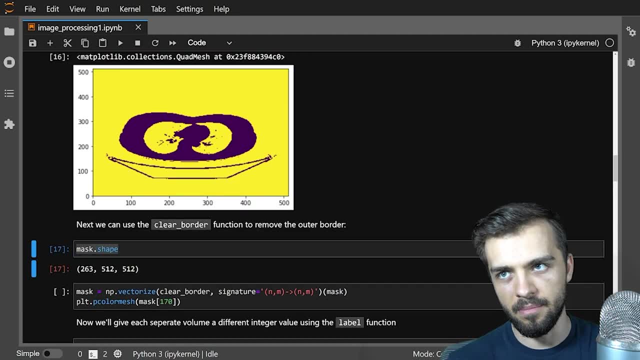 which takes in a 2D array, and it returns a 2D array And I feed in this 3D array mask. It's going to do it for every slice in the 3D image, which is the mask, and it will return a corresponding. 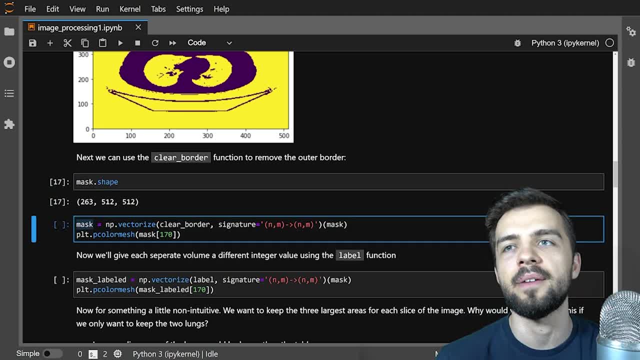 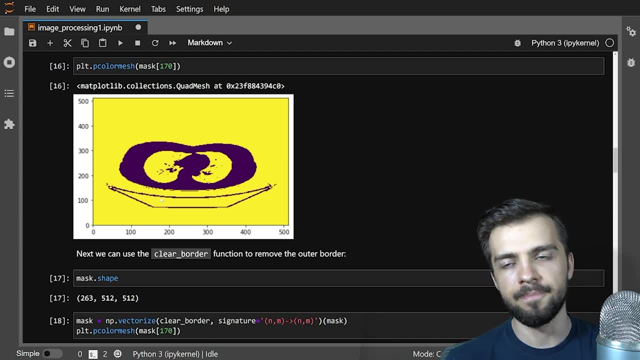 3D array, where I've applied this function to each slice of my array, And so I can do this. and then I can look at the mask, the same slice here, and you can see that it's taken this outer border and it's removed it, And that's exactly what we have here. So now we're going to do a little trick. 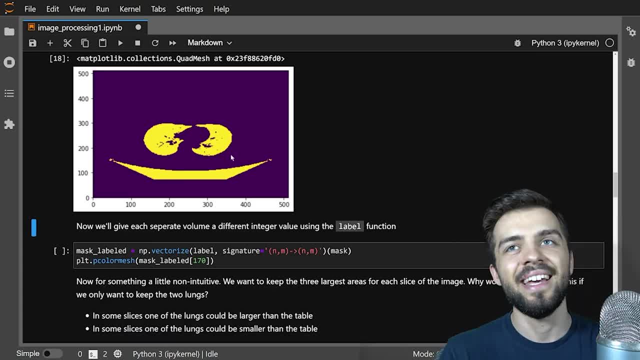 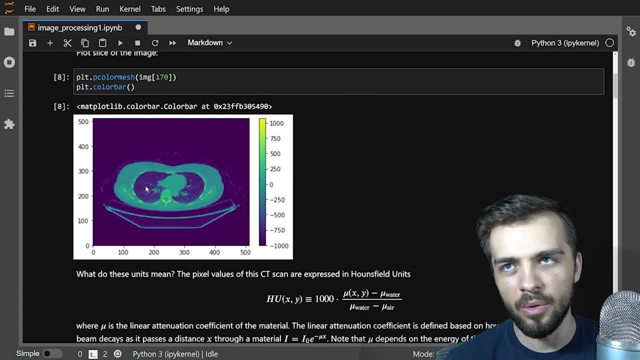 We have the lungs, but you can see the table also showed up. That's because the table kind of looks like a lung And you might think, well, no, it doesn't. But to the computer it's basically a hollowed out region of air. 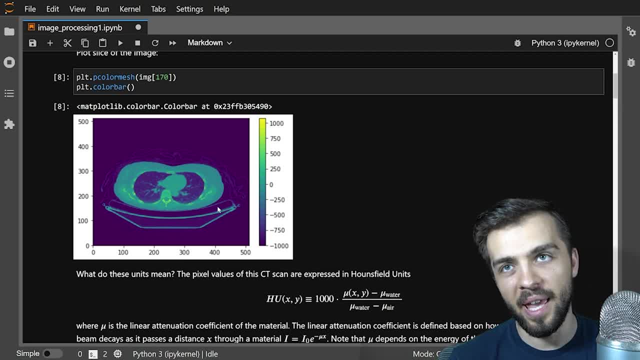 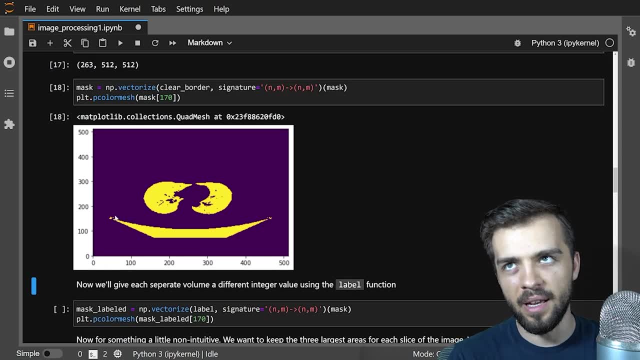 surrounded by high attenuation coefficients. So the table is a real pain actually for our challenge. The reason why it's a pain is in some slices. if I compare the area of the lung to the table, the lung is going to have a larger area than the table. But if I look at a different 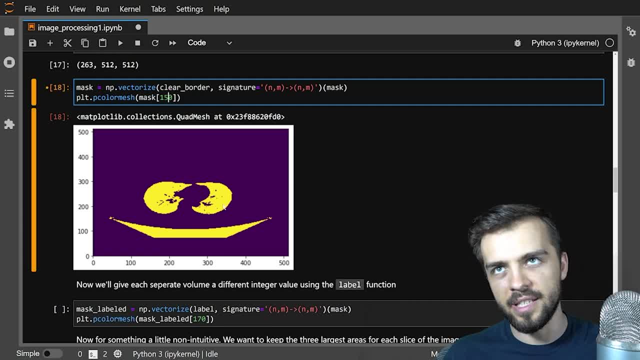 slice, for example here. so here the lung might have a larger area than the table. So if I look at a larger area than the table, but in a different slice, you know, for example, this is part of the lung, but it's clearly smaller than the table. So what we want to do is we want to create different. 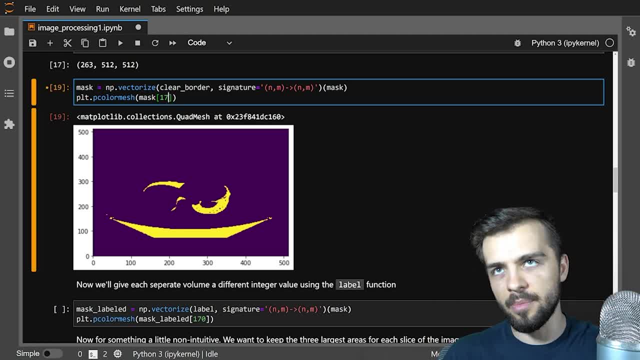 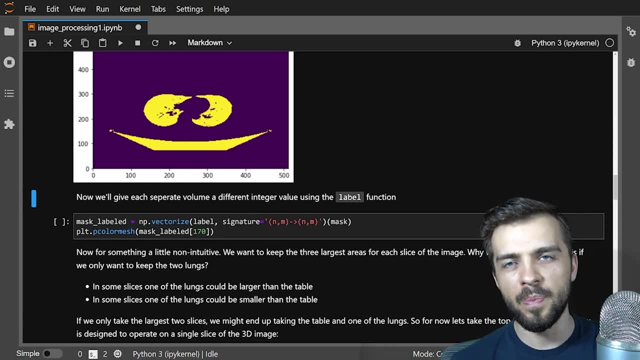 regions for each of the separate volumes in this image. that's going to be the first step to just selecting the lungs. So, for example, this might be region one, region two, region three, And for this we have the label function which we imported from scikit image dot measure. here it's. 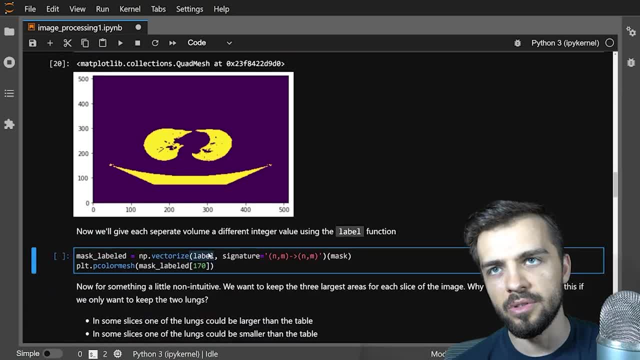 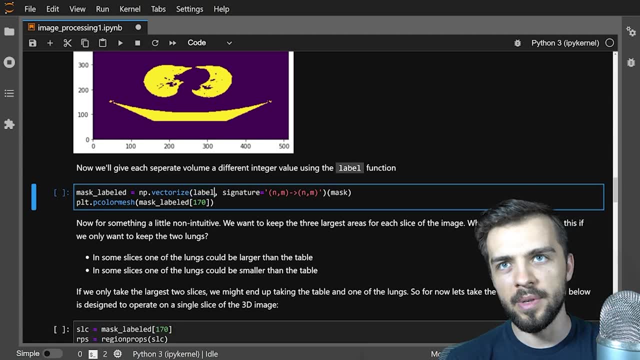 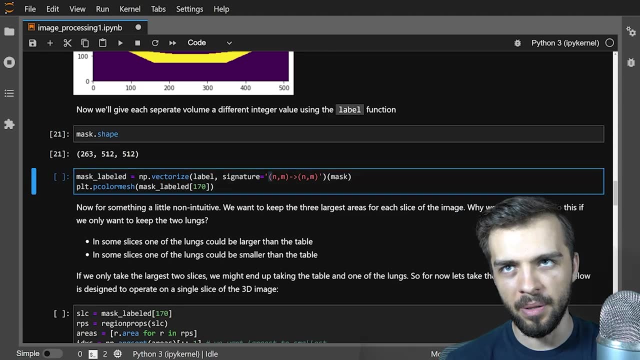 going to take a Boolean array where you either have ones or zeros, like this, And it's going to take each separate, distinct region and give it its own integer value. So what I'm doing is I'm calling it on the 3d array mask- remember that mask is a 3d array still- And I'm saying: Okay, you're going to apply this. 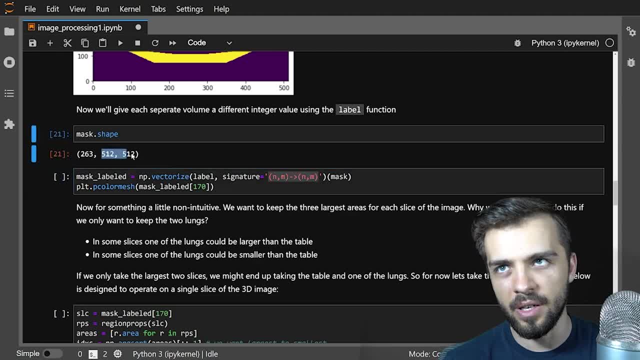 function label. it works on 2d slices. it's going to work on each 512 by 512 slice. it's going to loop over all these slices and return a corresponding 3d array which is mask labeled, And so I do this. 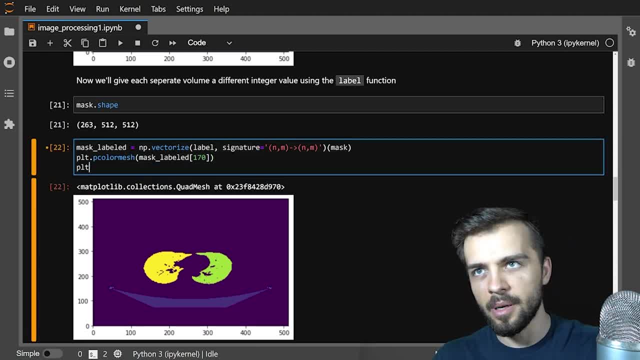 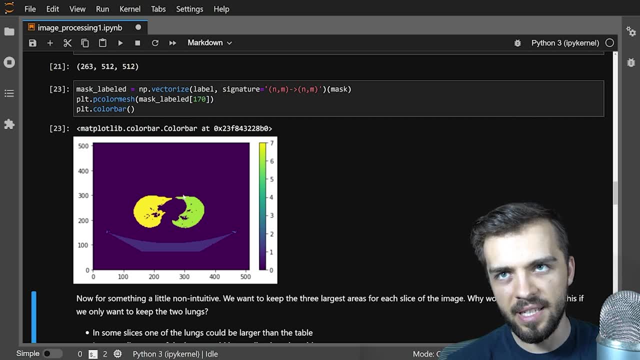 And I also want to see. you can see that I have different regions here And I'll give a little color bar just to show what's going on here, So you can see that like, for example, this has the integer value seven, this has the integer value six. there's a few other little areas that you can see. 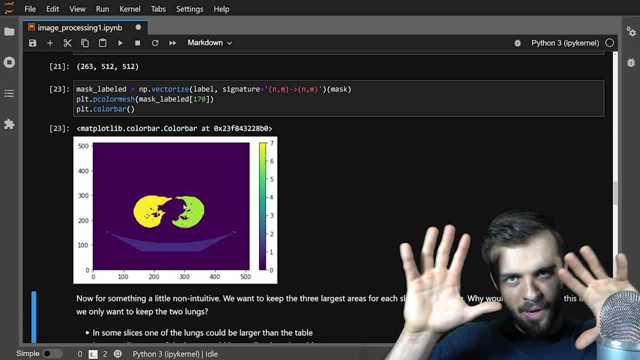 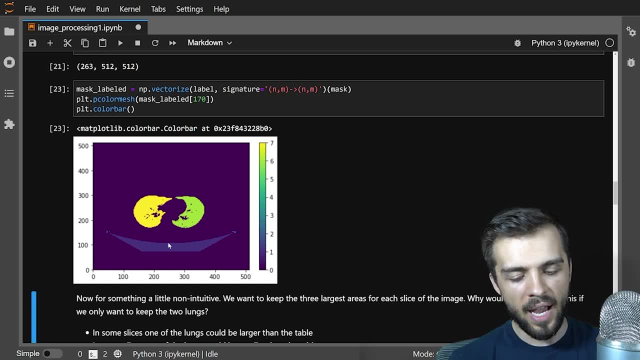 here that have also been segmented, and the tables like this. So I have all my regions in the image, given separate integers, And that allows me to differentiate between: Okay, this is lung, one lung to the table and I'll have integers corresponding to the different. 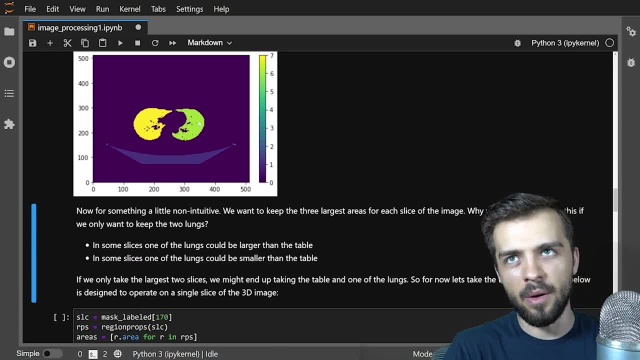 of the image. Now, the reason I'm doing this is because I want to keep the largest three areas in every slice, So I can delete these little areas here and these little areas here and I'm going to keep lung lung table. And you might think, well, why would I do that? Why would 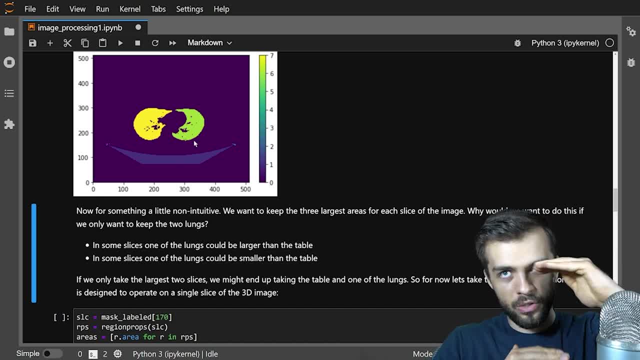 I keep the largest three areas. Well, remember, I'm doing this for all slices And, like I said before, in some slices one of the lungs is bigger than the table. for example, in this slice, But in another slice, maybe down here, you're at the bottom of the lung. The lung is going to be. 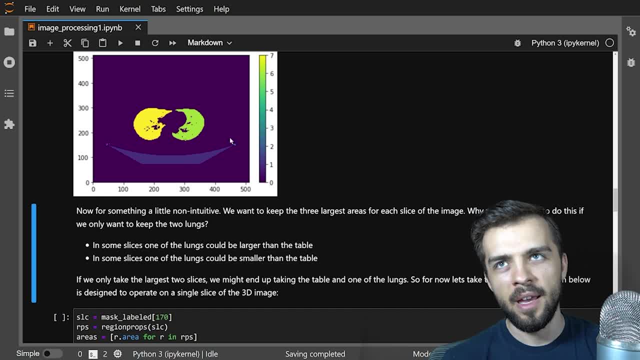 smaller than the table. So we'll deal with the table later. But the purpose of taking the largest three areas is I just want to get rid of any little areas. The table will be left, but it will guarantee that I keep the two lungs and then also, unfortunately, the table at this. 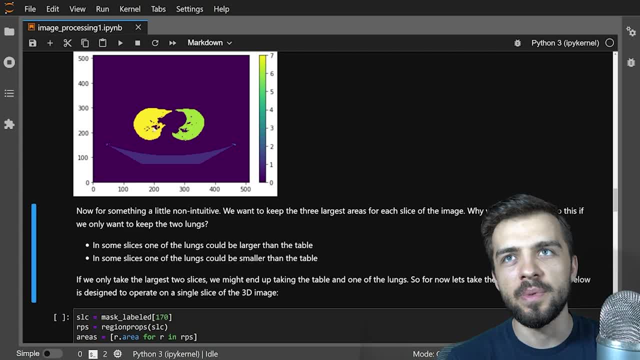 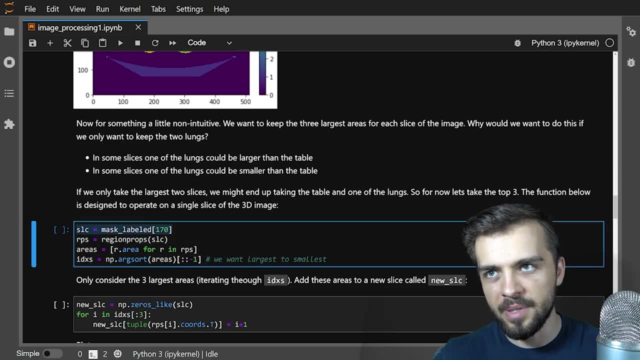 point. So how are we going to do that? Well, the first thing we need to do is we need to compute the areas of each of these separate regions, And so the way you do that- and I sort of go over that here. So here I'm taking a slice. That's basically the slice that I have plotted here, So I call that. 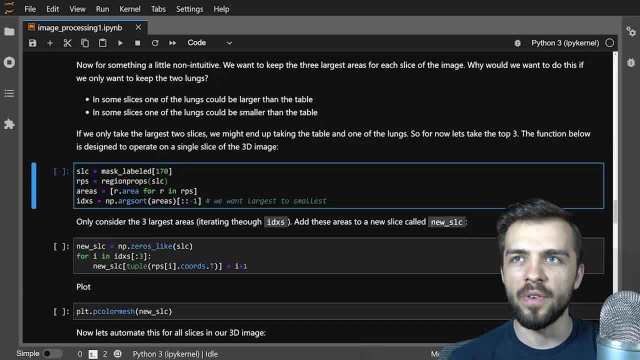 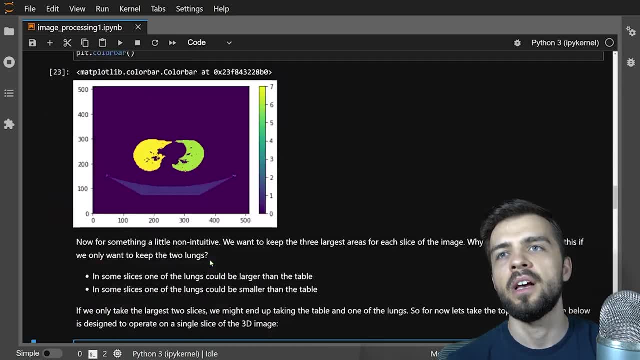 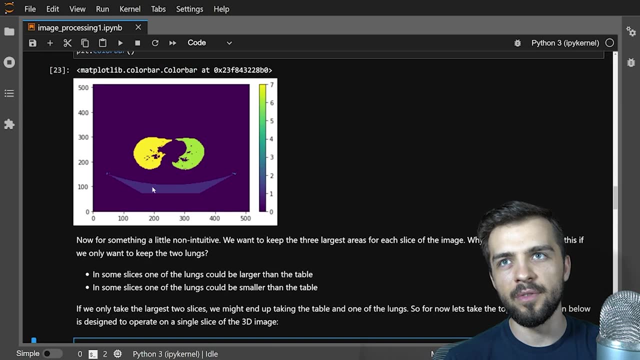 slice. Slice is a 2D array And then I can use this function called region props, which I imported above. Region props is from scikit-imagemeasure library. So what region props will do is it'll give the properties of each of the regions in this slice. So I have seven regions of this slice. 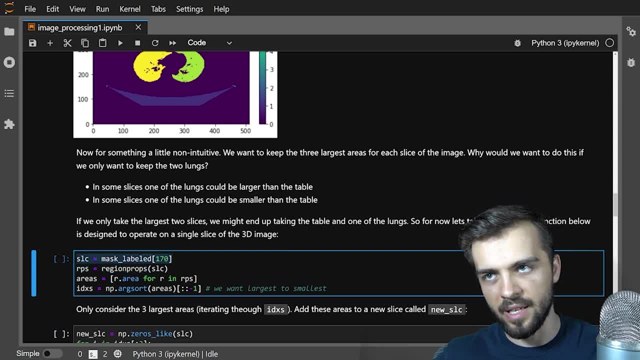 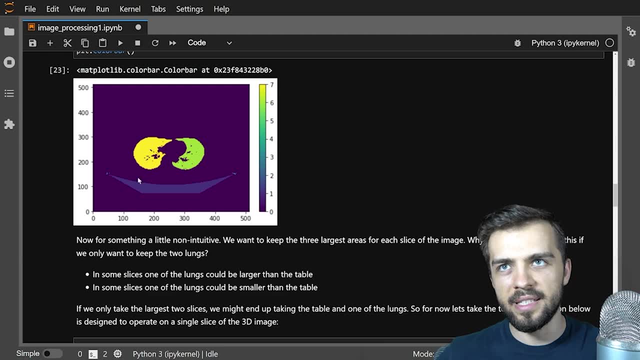 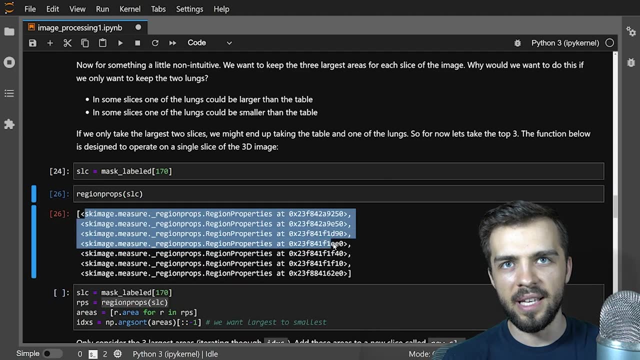 And region props is going to give me the properties of these, So I can just going through this slowly. Here's my slice. My slice is a 2D array. My 2D array is separated into different regions here And if I call region props on this slice, I have you know, a list And 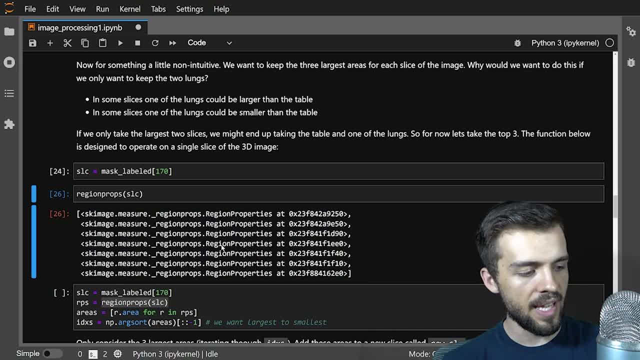 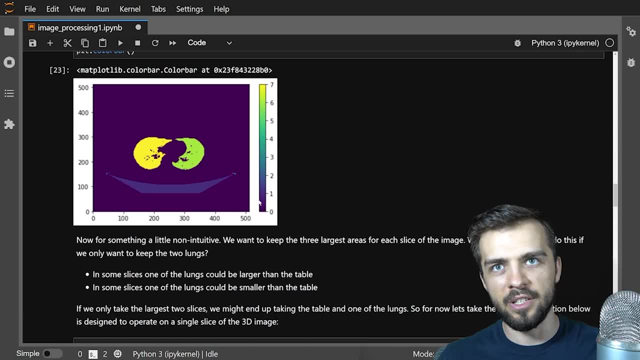 then there's different properties for each of these regions And if I want the area of each region, for example, I can call, for example, here's my first region prop. that corresponds to the region for the integer zero, for example, and I can call dot area will give me the area in. 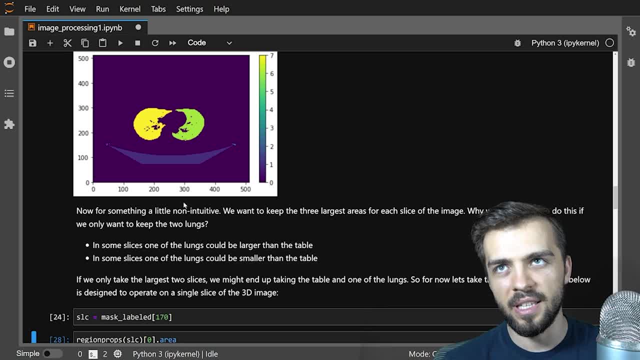 pixels of this particular region, of this slice. So iterate through all the region props, remember, happen a ray of the slice, So I'll iterate through all the region props, Remember I have. I'll integrate through all the region props, Remember, have an array like this, So I use a. 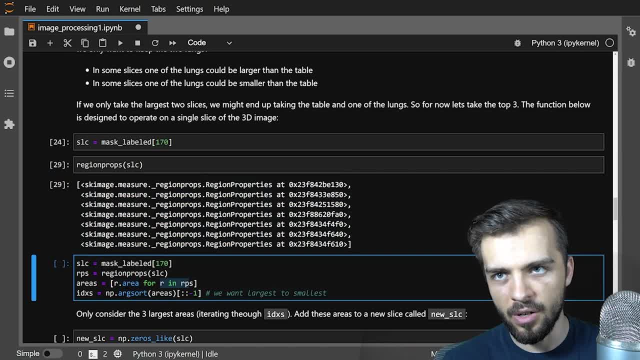 We want to know what is the Flensend습니까 here. Like I want to use pixels, let's say, if we get a list comprehension, I take R dot area for each of the R in the region props and that gives me my 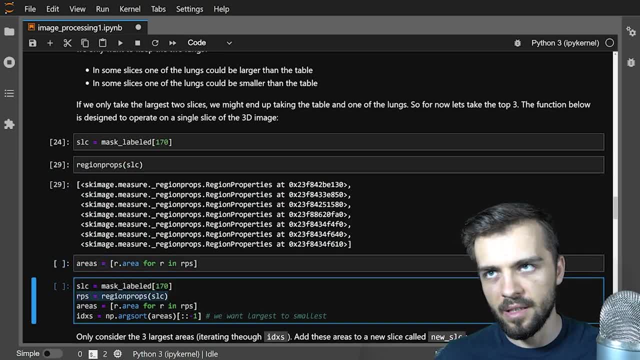 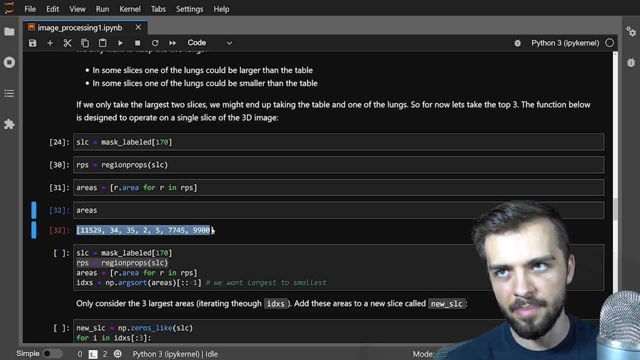 areas. so here I can set region props. is the region props of the slice? I get my areas. I can look like this and I have my areas of all the different slices and pixels. I have this sort of larger area and then these two sort of smaller areas here and then what I'm going to do remember. 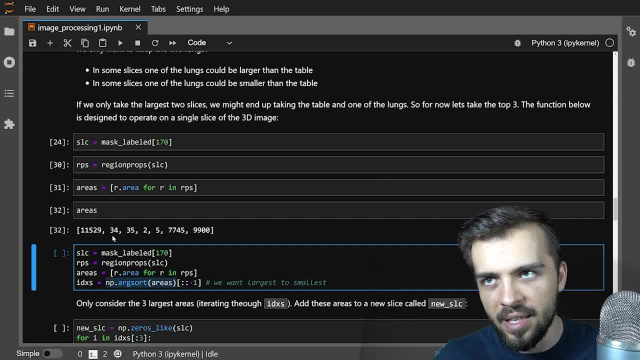 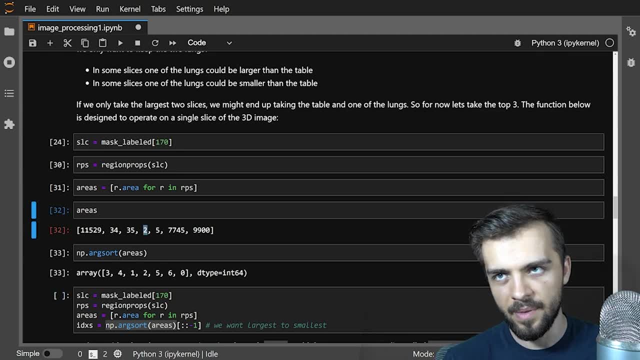 this is the areas. I'm going to take the areas from smallest to biggest. so index 3 is 2,. this is the smallest area. remember 0,, 1,, 2,, 3, this gives me my smallest index, 4, which corresponds. 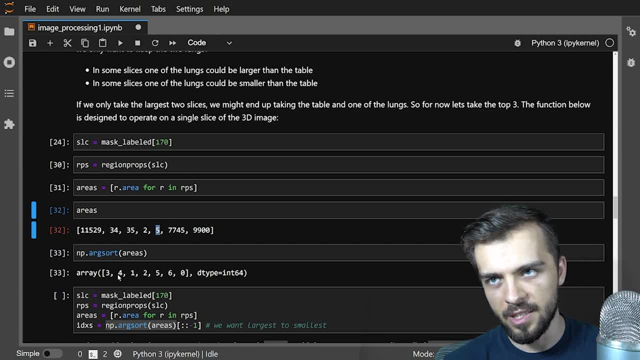 to this here: 0,, 1,, 2,, 3,, 4,, 5 is the second smallest, and then 34 is the next, then 35, and you can see that the indices are in order. and then what I'm going to do is I want from largest. 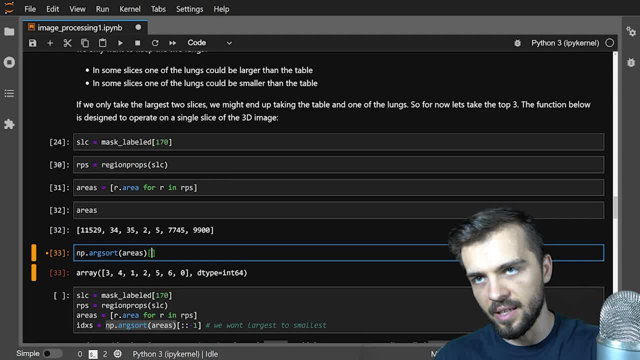 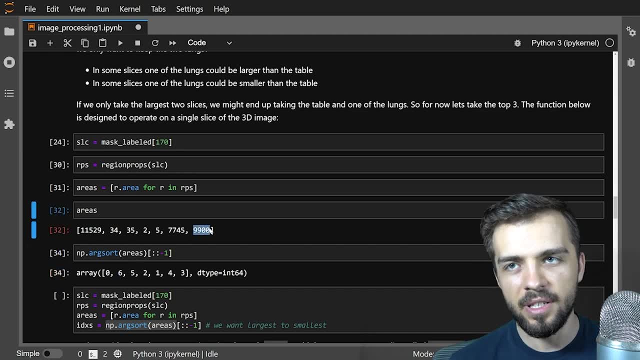 to smallest. So I'm going to take this backwards. that's why I give the two colons and the negative 1,. so 0 is the largest area, then 6,, 9, 900 is the second biggest area. so these are my list, of my integers. 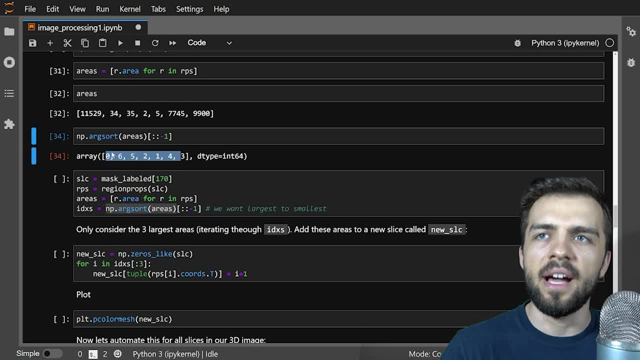 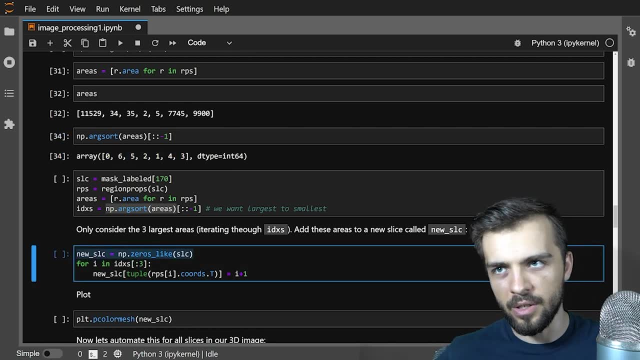 in order of biggest to smallest area. so I have these indices and now I'm only going to consider the three largest areas by looping through the indices. so the first thing I do is I create a new slice and I make it all zeros and I make it the same shape as slice. so my new slice is: 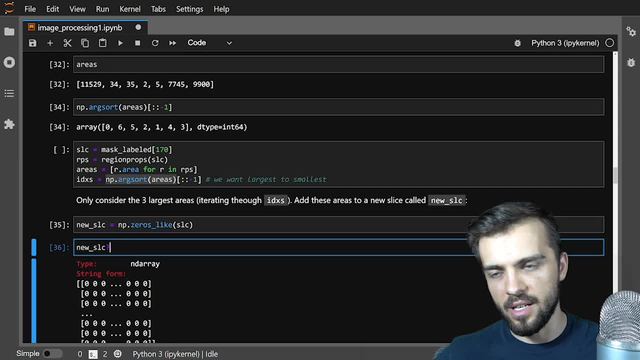 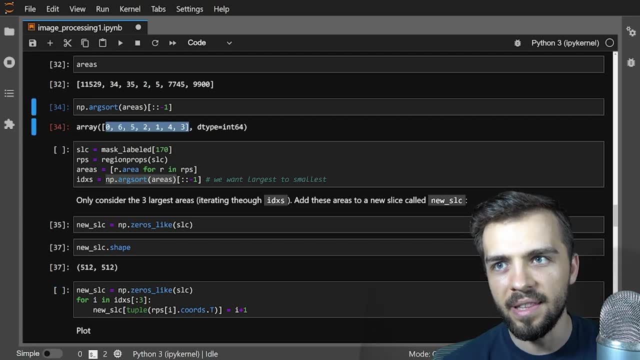 for example here: this is just dot shape, it's a 2D array, it's 512 by 512. for now I'm going to loop through these indices which I found above, like this and my new slice. here's what gets a: 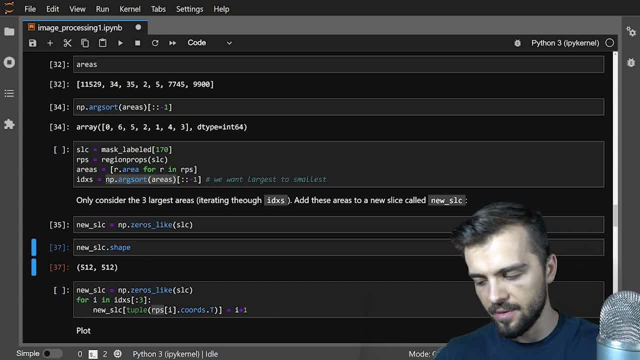 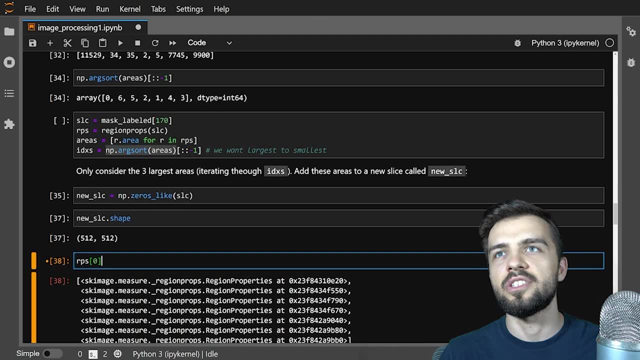 little tricky. I take my region props, which I have here region props, I take my ith region props. so, for example, here I could take my zeroth one. the zeroth region prop corresponds to the largest area. so I go like this: 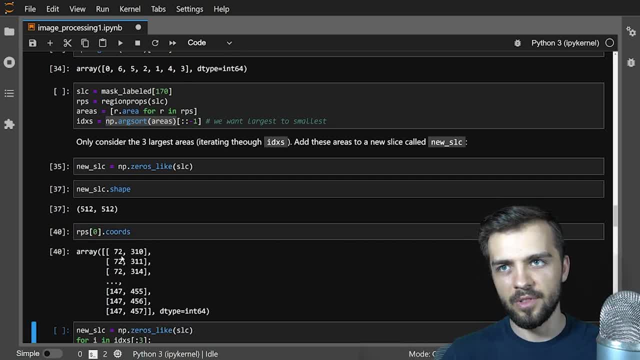 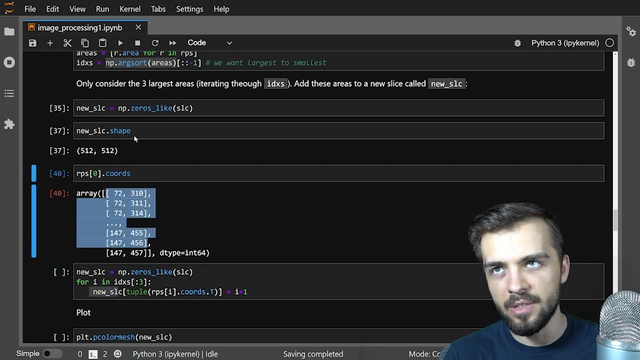 I can get the coordinates of this area like this. so here's my coordinates. now I want to get this in a way that I can index my new slice. so I want to index my new slice, which I created and I'm 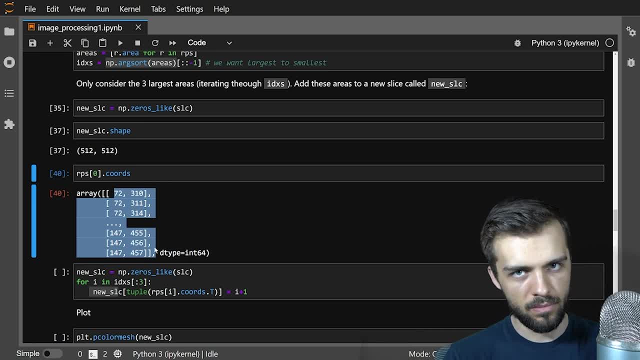 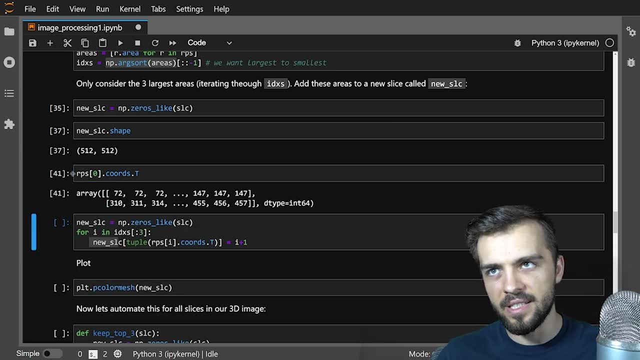 going to take out all these indices. I'm going to set it equal to 0, or 1, or whatever the index is. so here I have my things, but I need to. in order to do this, I need to transpose it like this: 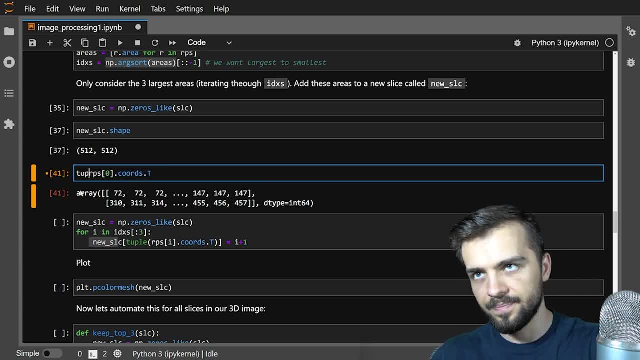 and then turn this into a tuple like this. So now I have sort of indices that I can index another array. then I take my new slice, which is 512 by 512, and I can index using what I created here, and now I have all my values at these points. 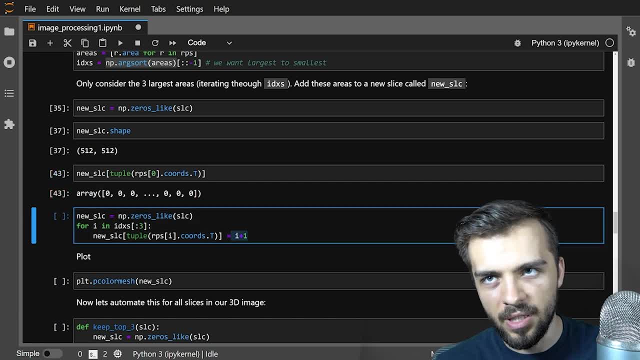 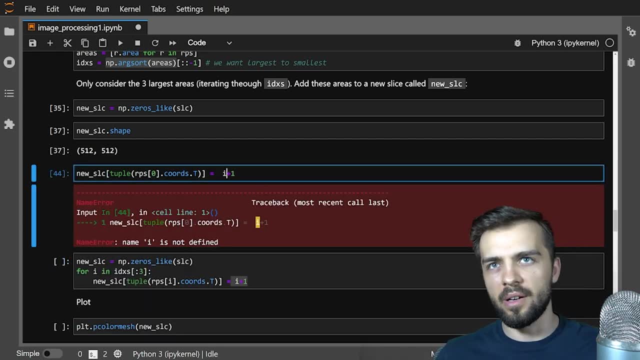 and if I want to set this equal to a particular value, I'm going to set it equal to i plus 1, so here equals i plus 1,. well, here I don't have i defined, but I could set it equal to 1,. 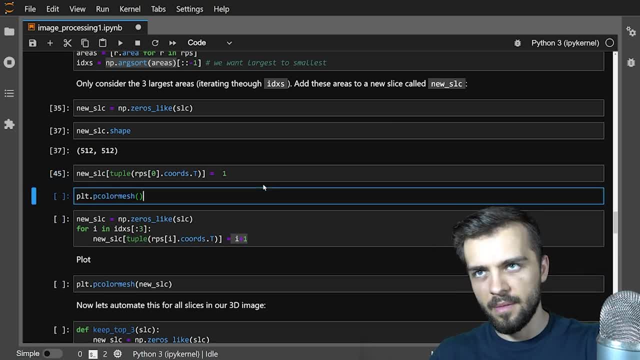 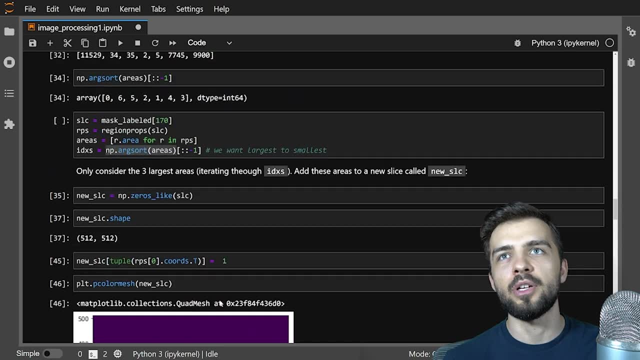 for example, and now I can plot that p color mesh, my new slice, and you see that I've taken this region and I've set all the values equal to 1, and I'm going to do that for the three largest areas here. so I create my new slice, I go through, 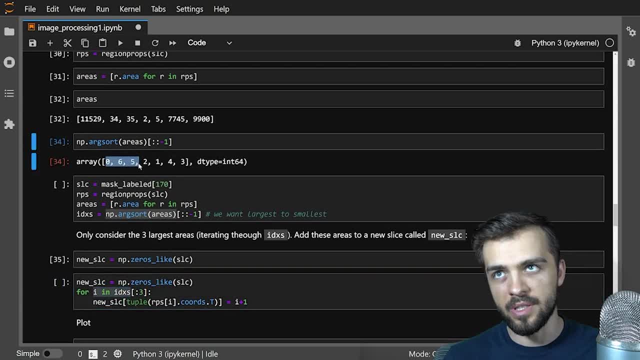 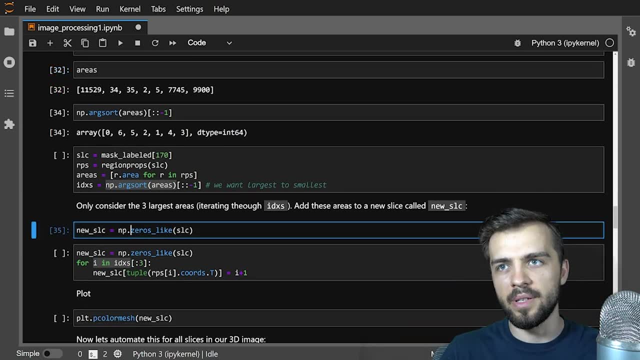 the indices corresponding to the three largest areas, which is going to be 0,, 6, and 5, this, this and this, each setting them to the corresponding separate, distinct integer. and that's what I do here and I don't know my indices defined. I have to run this, this. 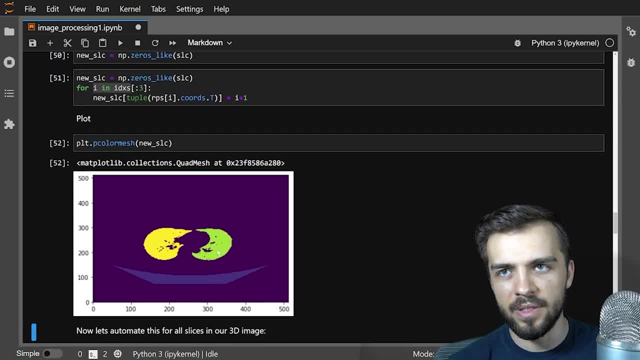 and then I can plot my new slice and you can see that I have three different regions here, each with its own color. I've removed all the smaller little areas. Again, we went through a lot of code there. you should sort of go through this, slowly, break it apart, like I did, And I think you'll understand. 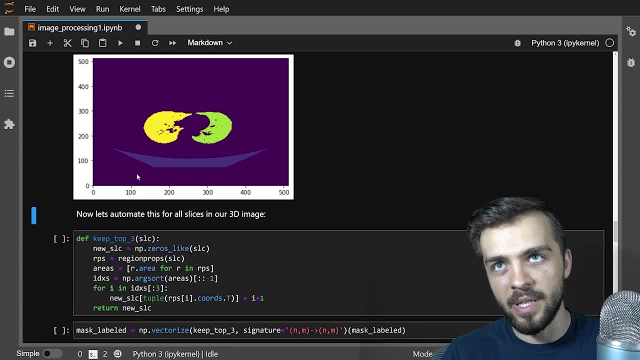 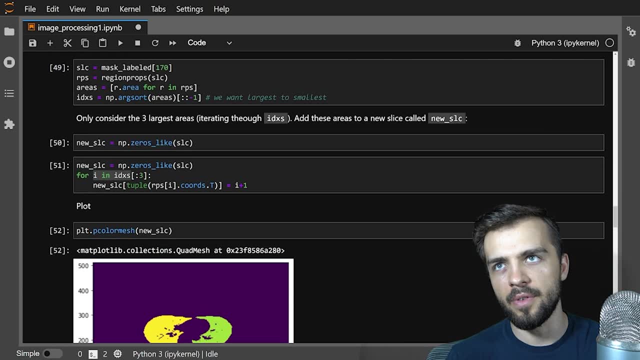 exactly what's going on here. So now what we're going to do is we're going to do this. we did this for one slice. we want to do this for all the slices in our image. So here's a function called keep top three. it's basically a summary of all the code we did above. we create a new slice. 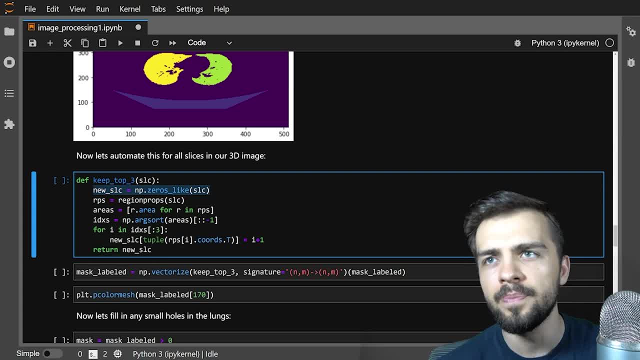 which is the same shape as the old slice, set equal to zero. I take the region props for that slice, the areas and the indices, and then I loop through the indices corresponding to the three largest areas And that new slice, which is all zeros. I set each of those equal to integer values. 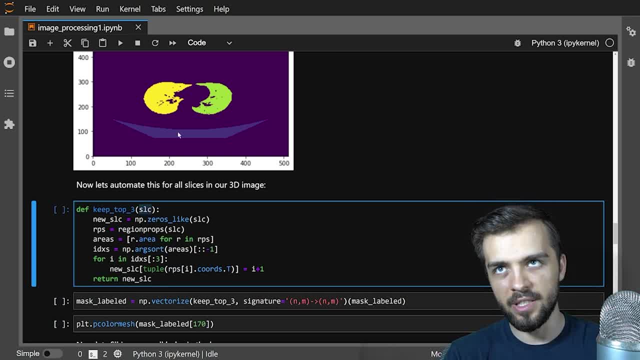 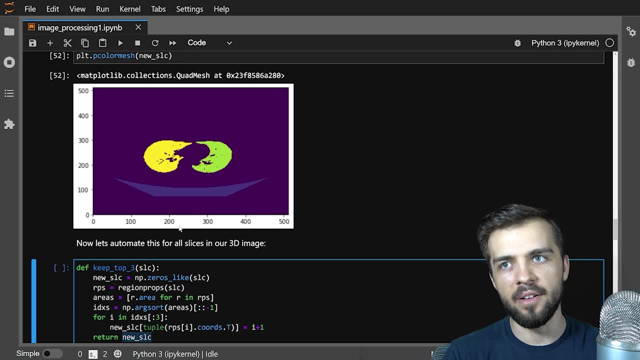 like I did above. So this takes in a slice, the old slice, which has all the different areas on it, and it returns a new slice which corresponds to separate integer values, the top three areas. because I have a function that does this, I can then vectorize it like I did before. 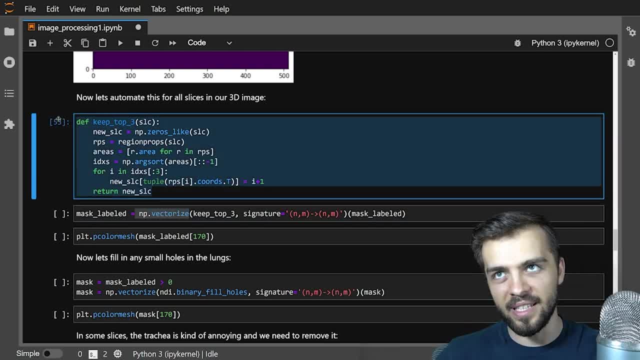 we'll keep. top three only takes in a 2d slice. that's how I defined it here. the top three, top three areas takes into 2d slice. but I'm feeding it a 3d array called mask, labeled And again vectorize. if I didn't give it the 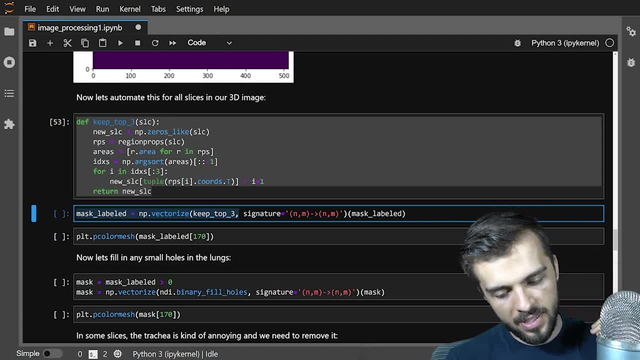 signature. it would try to go through every element of the 3d array, But I'm saying no. I want you to take in a 2d array and return a 2d array, And that's what you're vectorizing here. 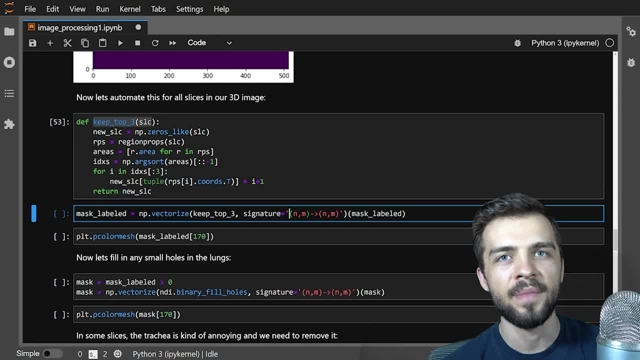 you're taking. you're vectorizing a function that takes in a 2d array, And so it's an nm to nm, that's 2d array in the signature. And it takes in mask labeled. it's using a 2d array and then it takes in a 2d array, And so it's an nm to nm, that's 2d array. 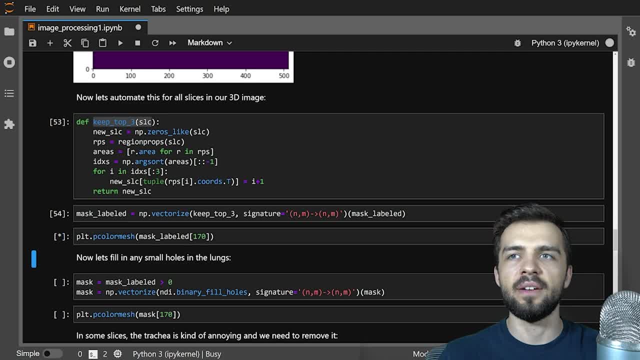 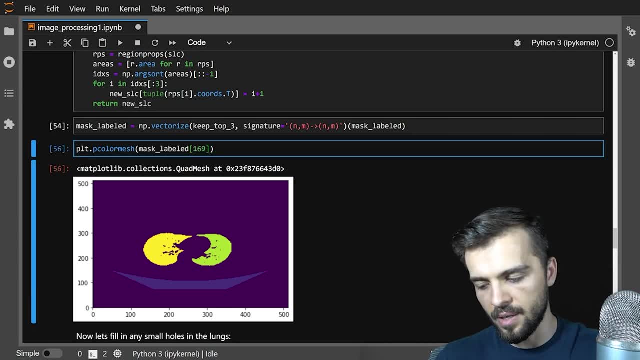 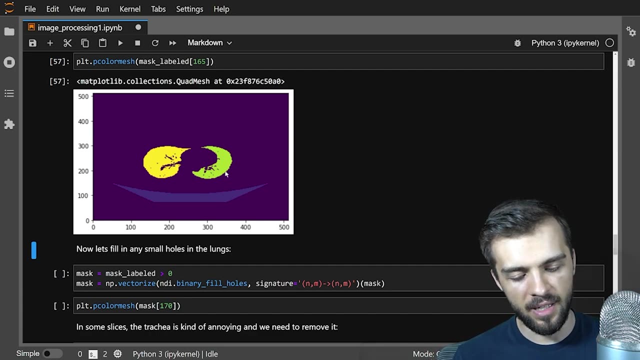 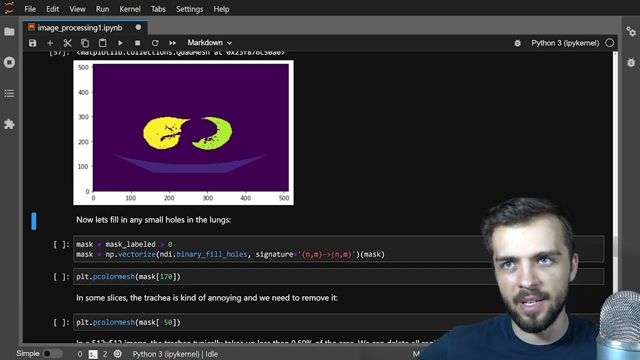 The next thing we're going to do is we're going to fill in all these small holes in the lungs. they're kind of gross and it's easy enough to do with these functions. So, first of all, I'm going to turn this back into a binary array where I just have separate areas. 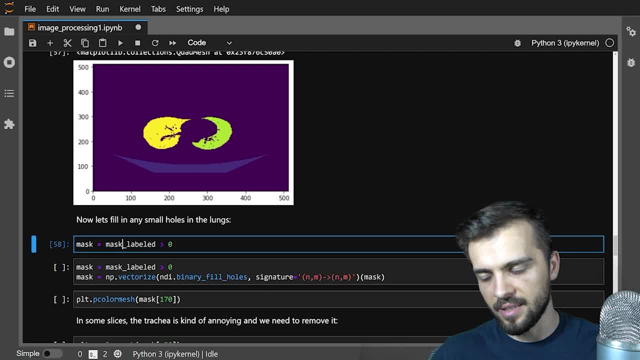 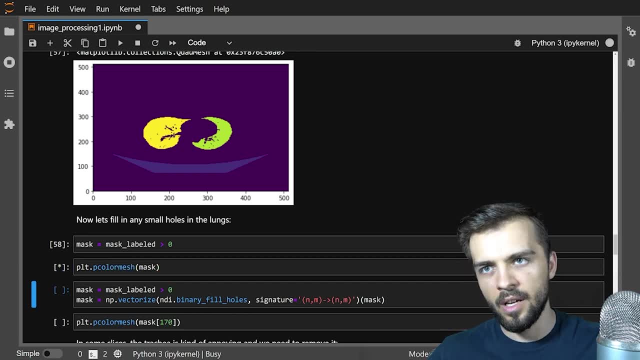 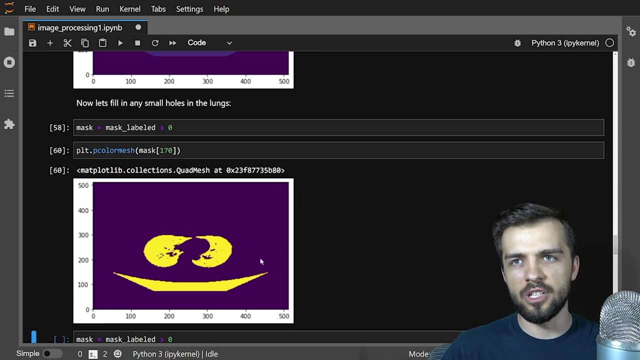 In order to do that, I just create a mask, And that's where a mask labeled is greater than zero. And, of course, if I plot dot p, color, mesh this again. this is a 3d array. this is not going to work, but I can give it the 170th slice And now you can see, it's just. 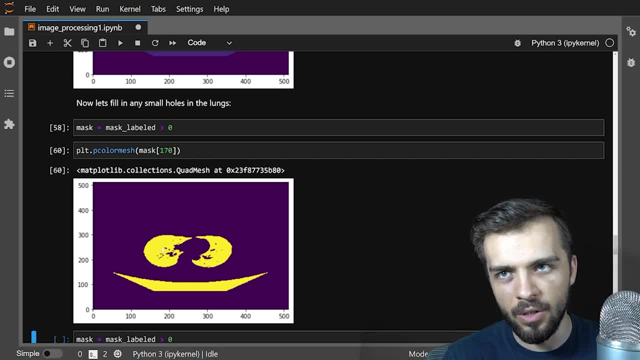 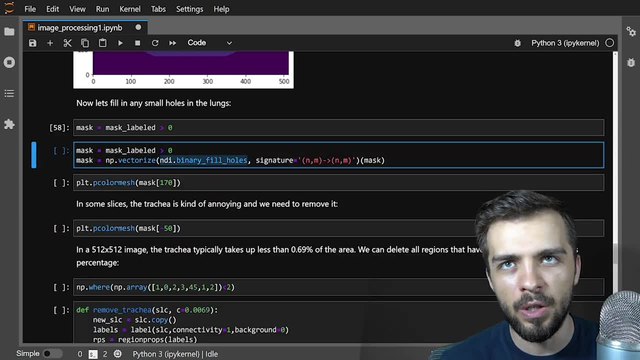 a Boolean array of ones and zeros, And what we're going to do is we're going to fill in all the little holes of this Boolean array, which is just trues and falses. For that I use this ndi dot binary fill holes function. Again, it's a function that takes in a 2d image that has ones or zeros and 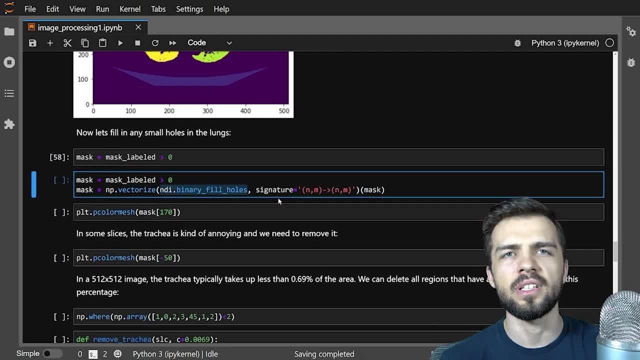 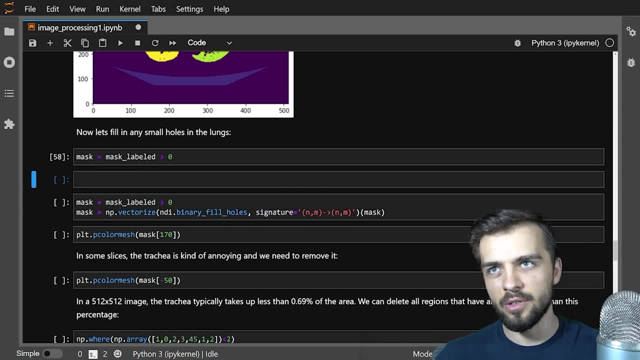 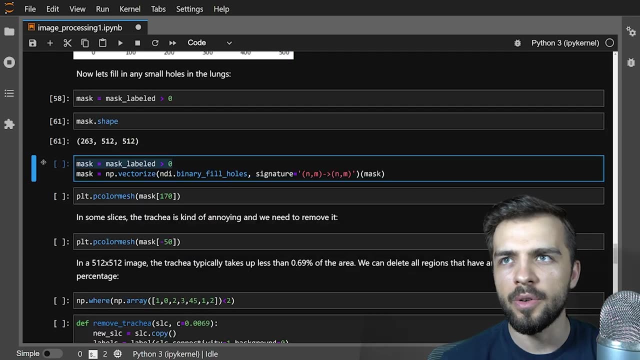 it fills in the little holes. this is sort of what the image looks like And I'm vectorizing it. So it does it for each slice in the 3d array mask that I give it because, remember, that mask is still a 3d array And I want to apply this to every single slice in that 3d array. So I create my mask And 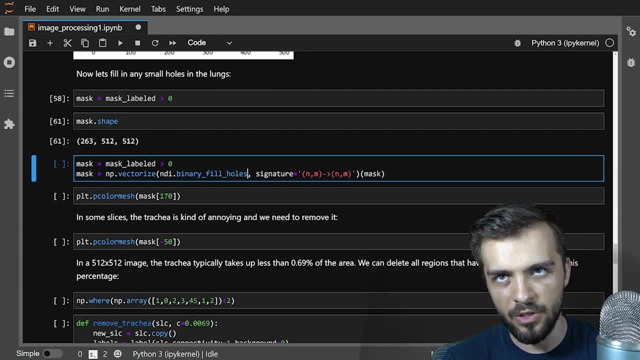 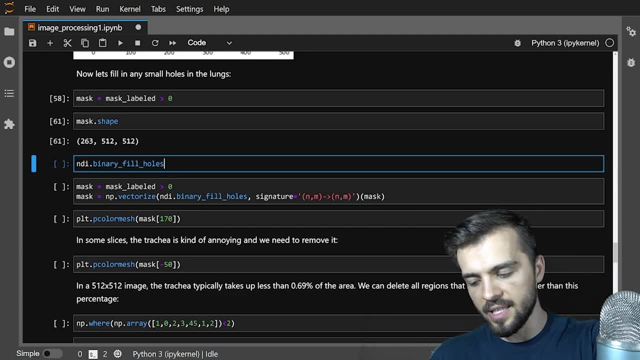 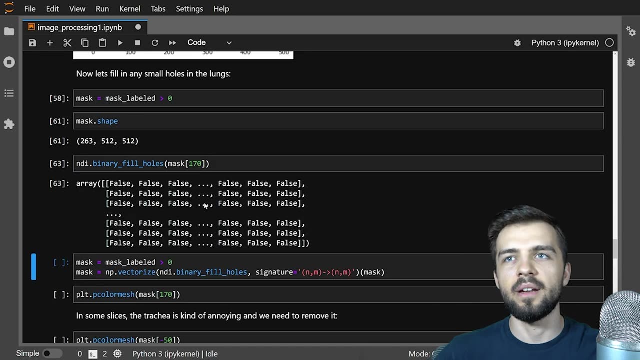 then I vectorize this operation which fills in the holes. So this is the function I'm vectorizing: binary fill holes. Again, if I wanted to, I could just call this function on a slice of the mask, mask 170. I can type here: ask 170. And it will do this automatically. But here I'm saying okay. 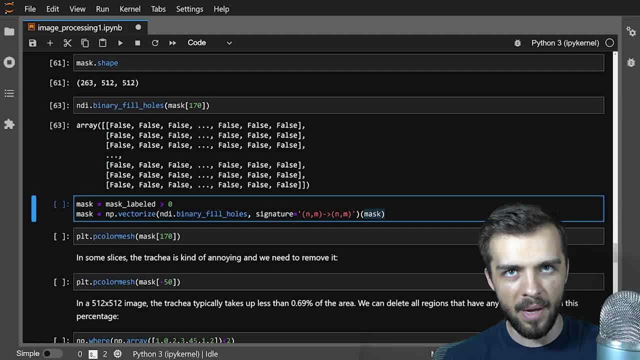 I want you to vectorize this function And I want you to do it over the full 3d mask but only on 2d slices, 2d slice by 2d slice, So it'll go off the first axis there of mask. So mask dot shape. 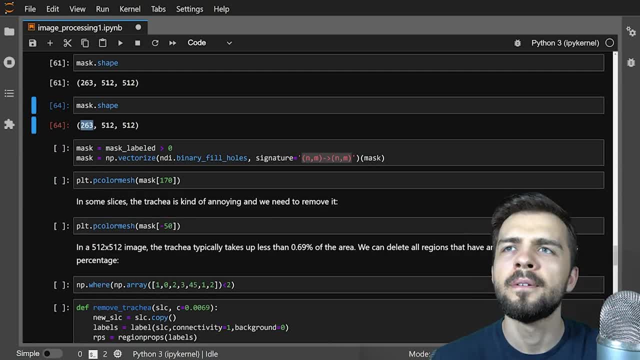 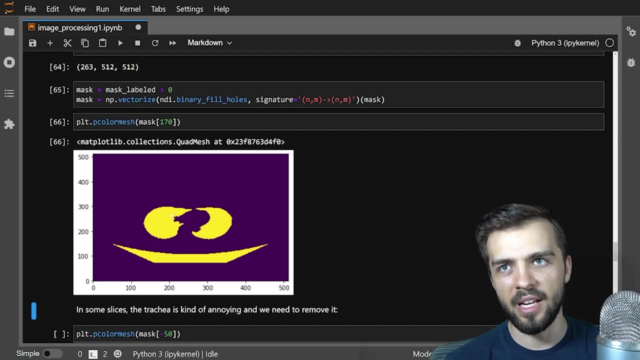 it's going to do it for all 263 elements. So I get my mask. this will fill in all the holes and I can plot that color, mesh it And you see that I've gone from an image that has sort of holes in the lungs up here and now the lungs. 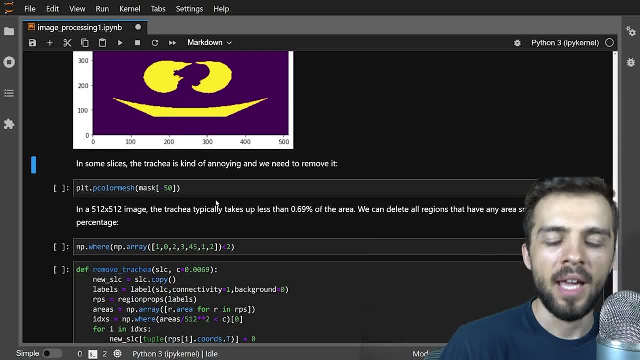 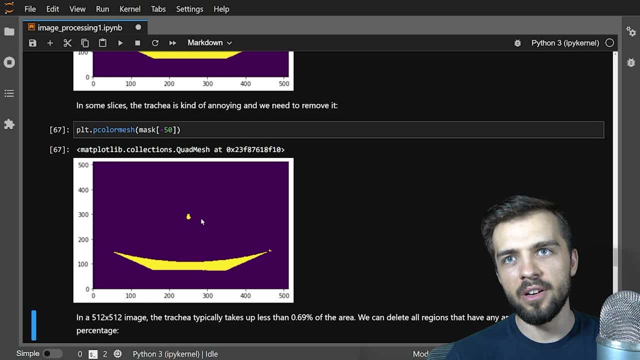 are nice and filled in. Now in some slices actually, you end up taking the trachea and it's sort of annoying. So if I look at this, for example, here sort of I'm above the lungs but I'm looking at a slice corresponding to the trachea and I have a hole here And I don't want. 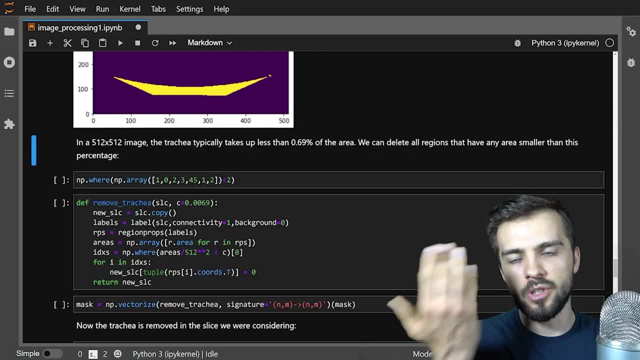 that hole. So we need a way to remove the trachea. So it turns out then in a 512 by 512 CT scan the trachea typically takes up a lot of space. So I'm going to go ahead and do that And I'm going 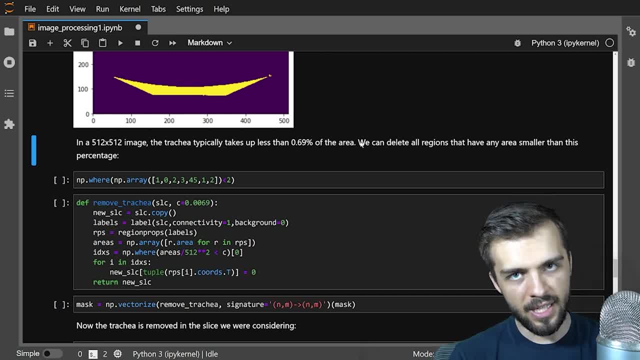 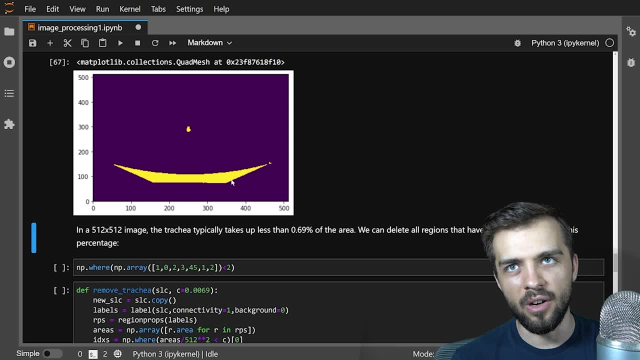 to go ahead and delete all the areas that have less than 0.69% of the area. So what we do is we delete all areas that have less than 0.69%. So again, I can use my region props function to take. 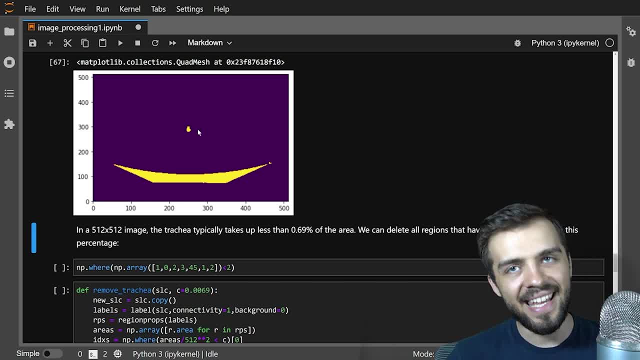 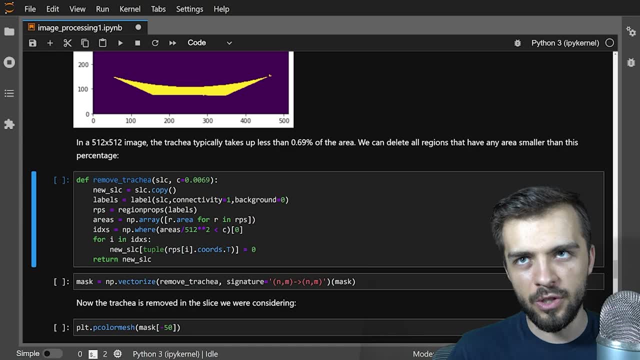 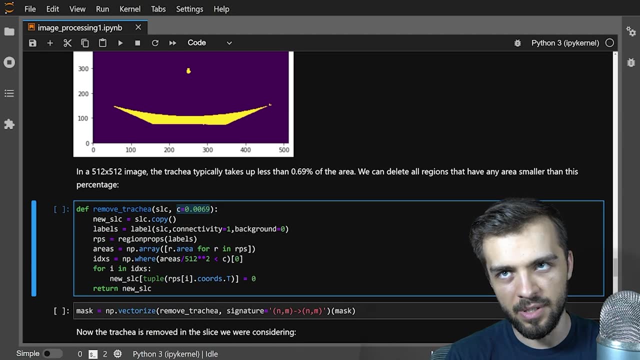 all these, separate three biggest areas and delete any areas that are less than 0.69% of the total area of this slice. So here's my function that removes the trachea. I take my slice and see which is the sort of amount of the area that it needs to be. less than is 0.0069.. 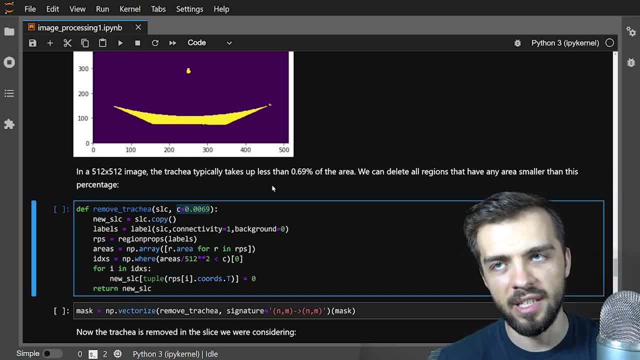 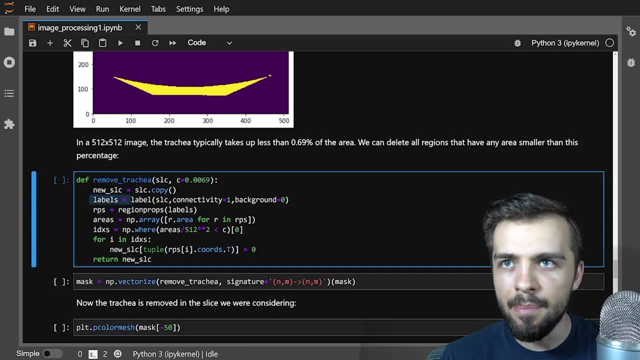 times the total size of the image: 0.69%. So here's my new slice. I copy the original slice of the 2d array, a slice like this, then I labeled the slice. This is like what I did before, So I 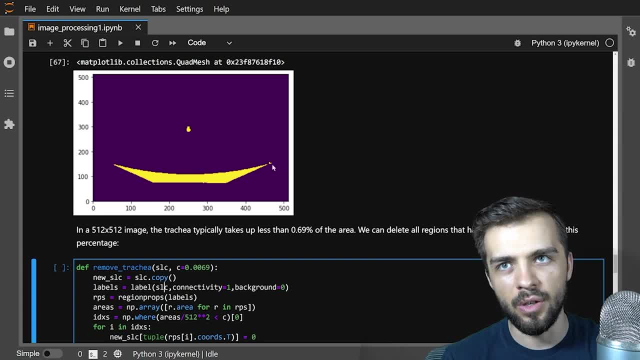 labeled the slice, So each of the separate areas will have their own label to them. Then I get the region properties of each of those labels, like before. So there's three different areas here because I've enforced that it's only the top three So I have here. it will give me the 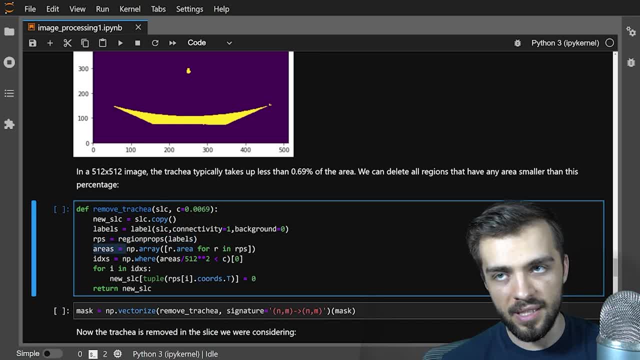 properties of each of these three regions. So I'm going to go ahead and delete all of these three regions. I get the areas, like I did before, And then my indices. now we're going to be well. I want to look at the location where these areas are less than C, So 512 squared divided by the areas. 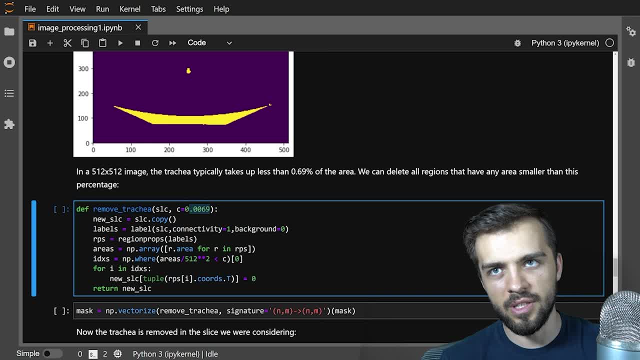 that's sort of the percent of the image, And if it's less than 0.0069, that would be like the trachea- then delete it. So we're getting rid of any small areas here in the image And that's. 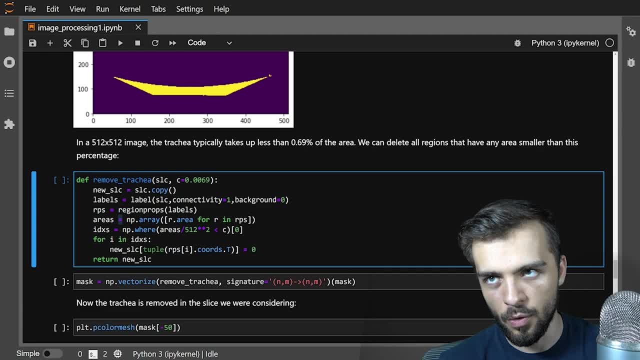 typically the trachea here. So these are the indices corresponding to each of those separate areas. Then I loop through these indices and at that new slice the locations where corresponding to those areas, we set those equal to zero and I return the new slice. So going through this slowly, 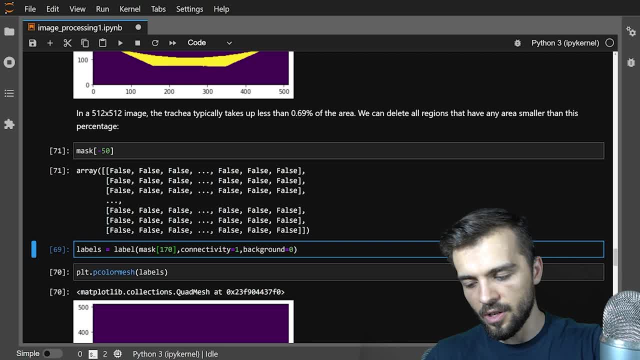 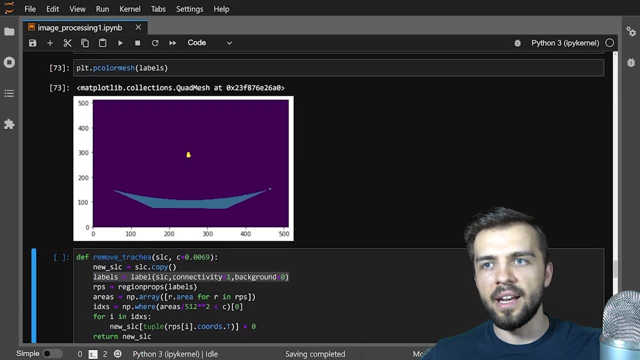 here's mask negative 50. I can call the label function on mask negative 50.. Like before, and I get this. So I have region one, region two, region three. then I call my region props on this, like before, and it should be an array of size three that gives me the. 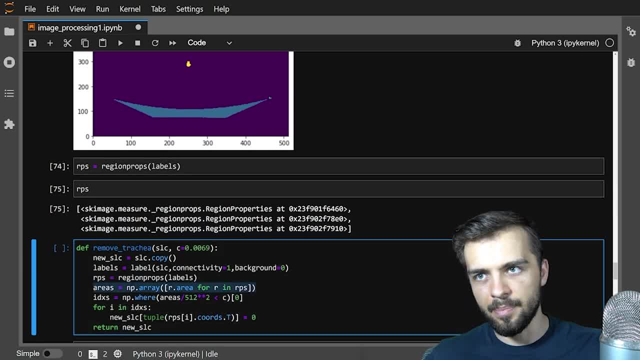 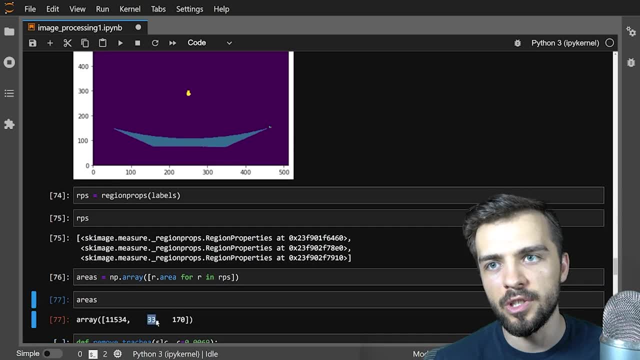 properties of each of these three separate regions. I can then get the separate areas for each of these regions And then I can look at the areas and you can see that one of them is big. That's the table. The other two are small and total area of pixels. Those are the other two. 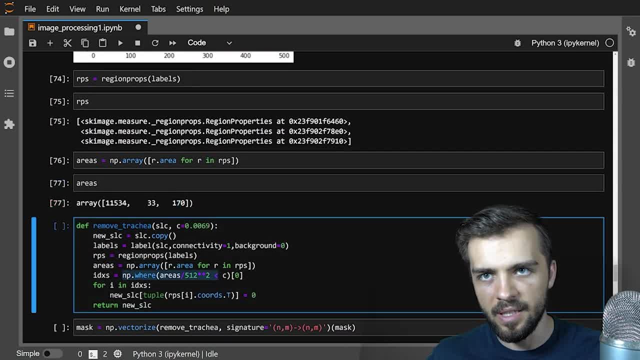 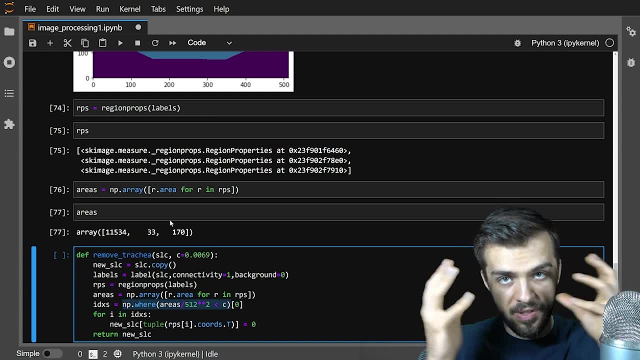 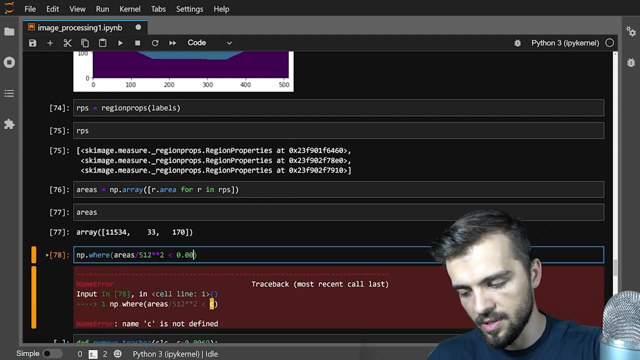 regions. And then I can look for the indices where the area divided by 512 squared is less than 0.069, which is the percentage of the image that we're using as a cutoff. So if I look at this 0.0069, it says that at indices one and two this holds true. And then I loop through these. 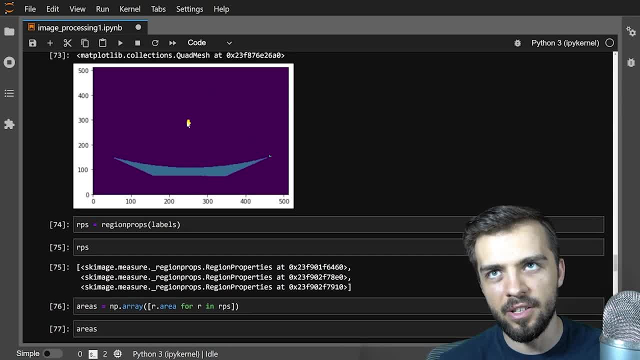 indices in my new slice set it equal to zero. So these areas are manually going to be set equal to the background value, which is zero, And then I'm left getting rid of all any small areas in this image. So here's my function. I vectorize this function because again, I'm going to pass. 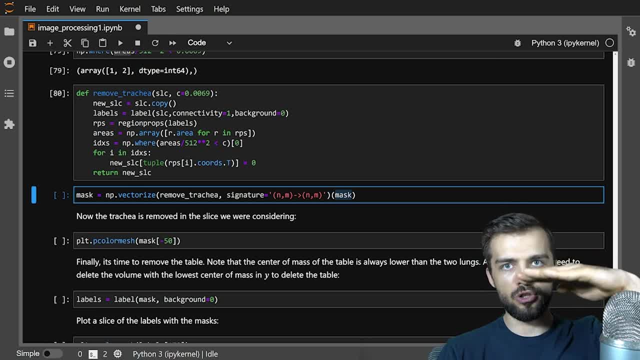 the full 3d mask in, but I'm only operating on each 2d slice of the image And it will return. remember, it takes in a 2d slice, it returns a 2d slice and it returns a 2d slice. So I can. 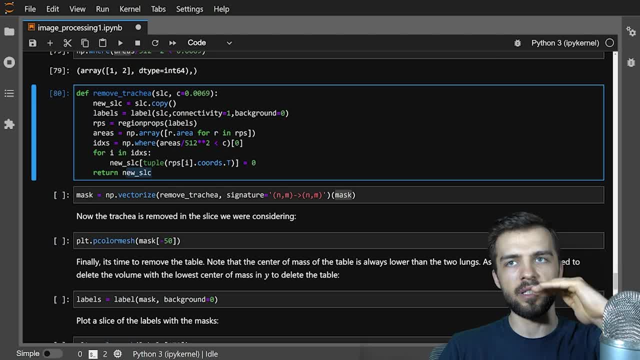 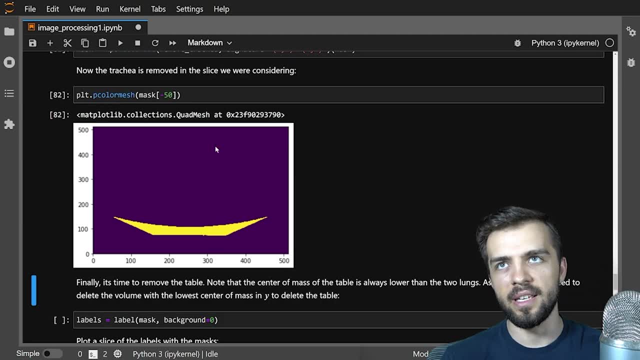 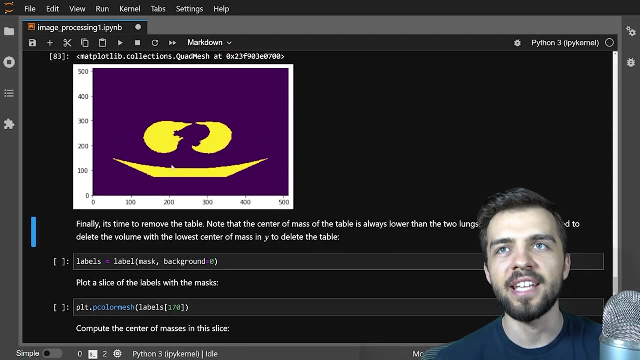 do this for all 263 slices and return a corresponding 3d array, And so now I have a new mask, And if I look at this, you can see that my trachea is indeed removed in the slices that I want, And everything else before is like normal. So now it's time to remove the table, And we're. 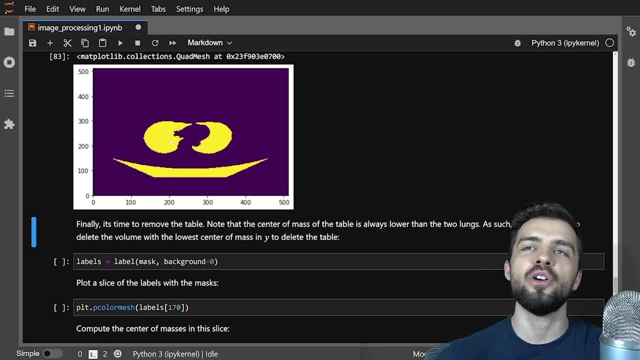 going to use a clever little trick here to do this. Now you'll note that each of these separate regions has its own center of mass. this is something from physics, And you can think of all these little pixels and you can see that each of these regions has its own center of mass. 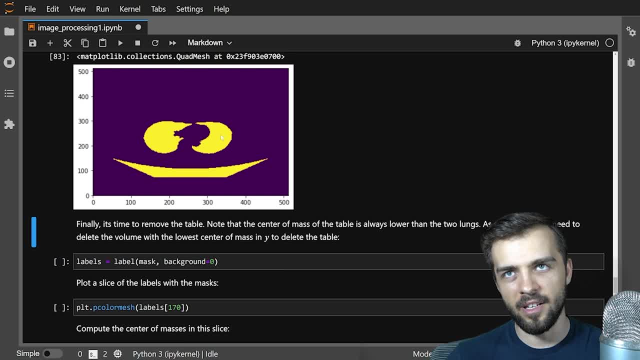 So this center of mass might be here, this center of mass might be here, and then there's one here. So what we're going to do is we're going to delete the area that has the lowest center of mass in y. that's sort of one way to think about this. So let's take an example. So 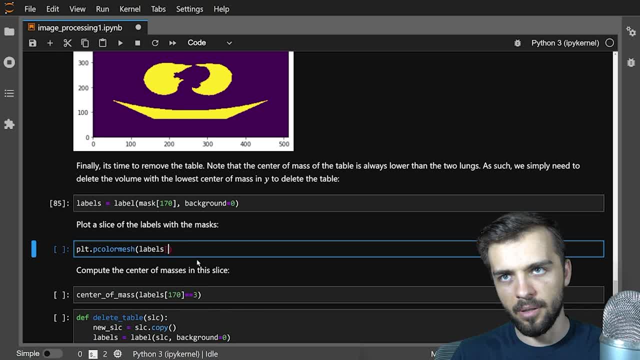 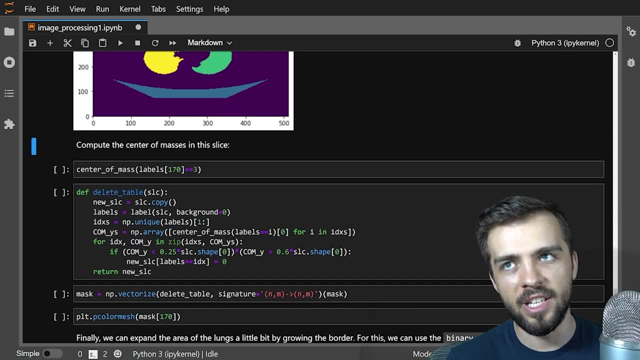 here's my labels, like I got before, and I can plot dot, color, mesh the labels like this And we can compute the center of masses for each of these separate regions. So I can call the center of mass function. I'm going to take one of these regions. So if I look at the 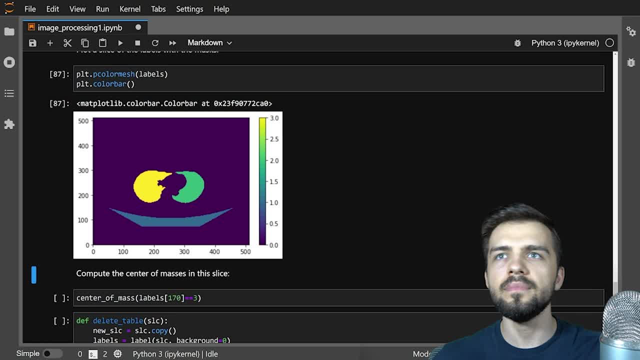 top plot dot color bar. here you can see that this corresponds to the integer three, this is the integer two and this is the integer one. the purple is zero, the background. So what I'm going to do is I'm going to say: Okay, let's look at the binary array where labels equals, equals three. 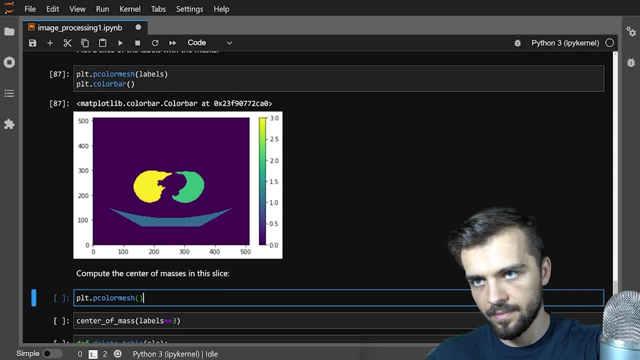 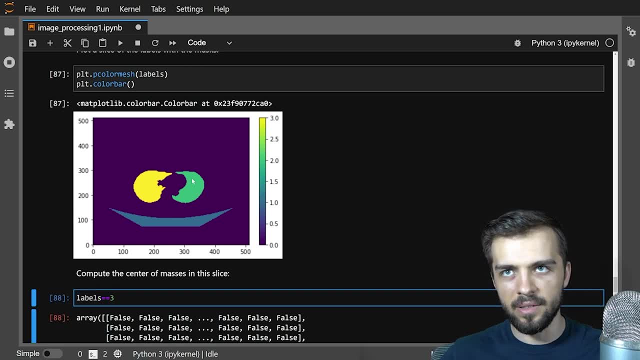 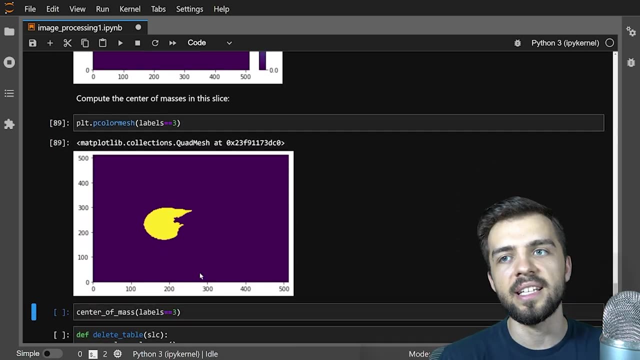 I can plot, dot, peak, color, mesh this, Remember this just gives a boolean array: labels, equals, equals. three is a Boolean array, So it'll be one are true here and then zero everywhere else. So I can color, mesh this and it gives me this thing here: from this 2d slice i can compute the center. 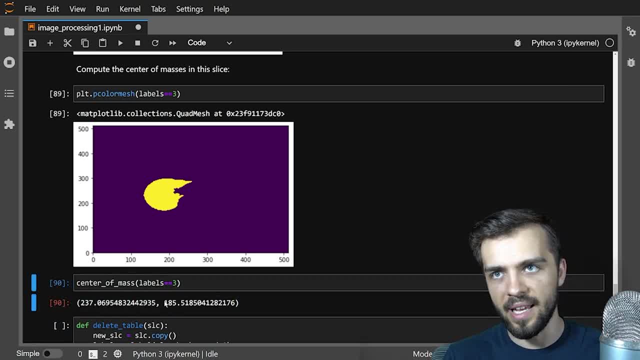 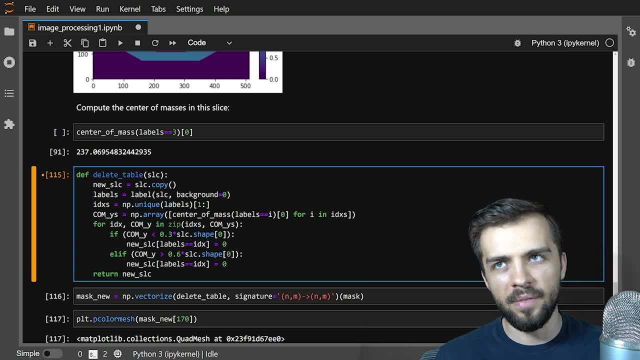 of mass and it tells me where it is in y and x. so 185 in x, 273 in y, here on this image. so now we have the delete table function. it takes in a 2d slice. the first thing we do is the. we copy the. 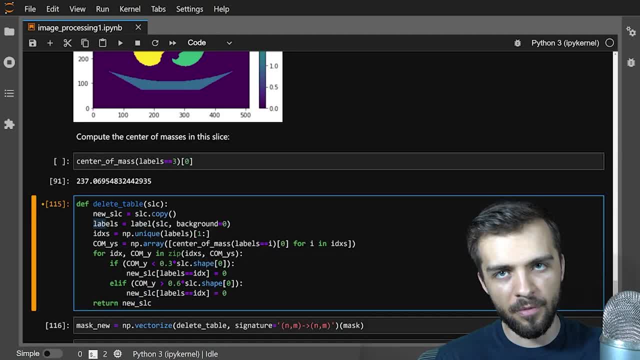 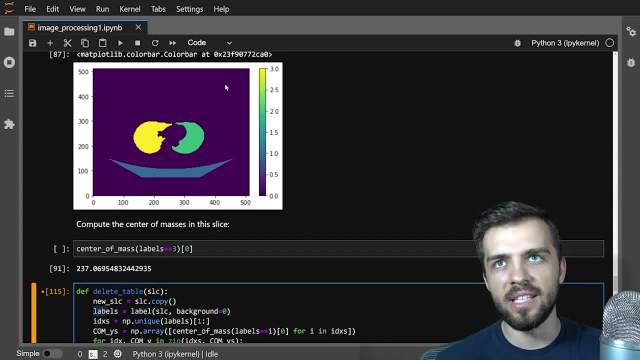 slice, then we label it like we did above. the slice is going to come from the mask and so it's going to be either ones or zeros. we'll label it to have separate regions like this: i will take the unique indices that are not equal to zero. so we go labels: the mp unique of the labels here, but uh, indexing. 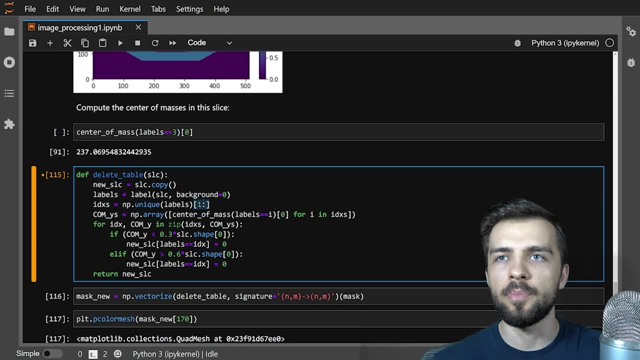 from one onwards, because we don't want to take the background. then we'll compute the center of mass for each of these- uh, separate regions and then what we do is we loop through the corresponding index, so whatever value is given to that region and the center of mass for each of these things, 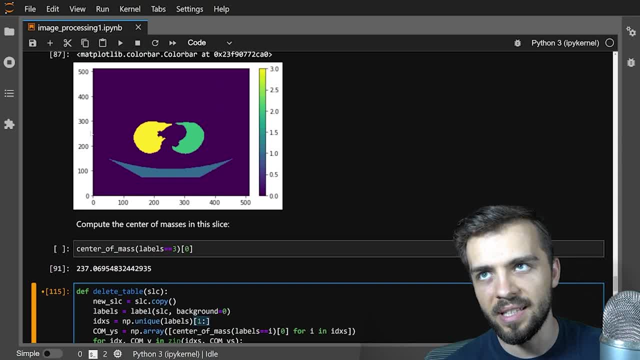 and i save the center of mass and y is less than 30 percent the height up here, delete it. so that will delete the table. and then also, if the center of mass is greater than 60 percent the height, delete it. the reason for that is sometimes you get the nasal bridge, which has air in it as well, so you get a little. 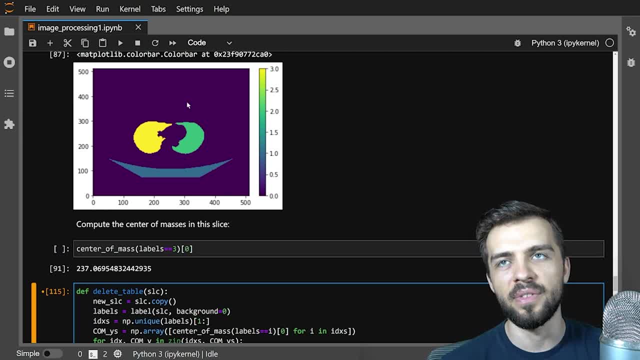 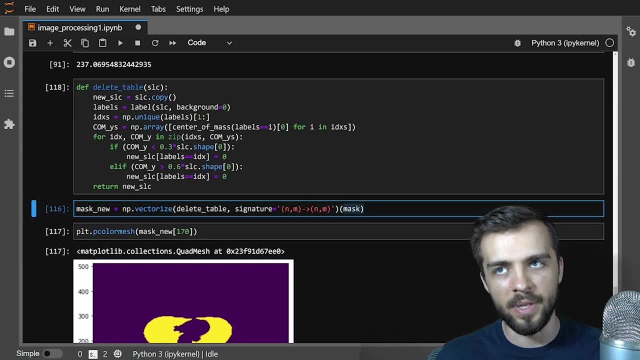 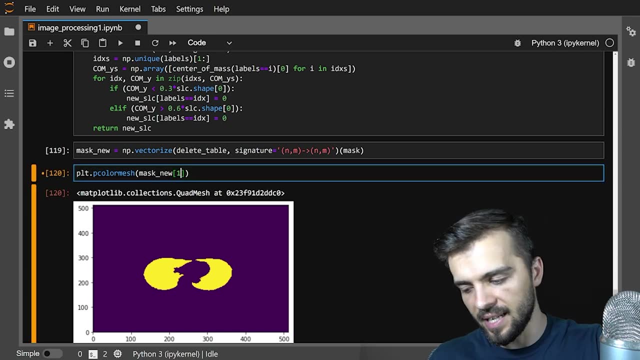 air pocket up here so that will delete any nasal bridge sort of thing here just to keep the lungs, and so i can run this function. we can create a new mask from our old 3d mask. then we can look at our new mask and, as you can see, the table is deleted, and it is deleted for all slices here. so this is beautiful. 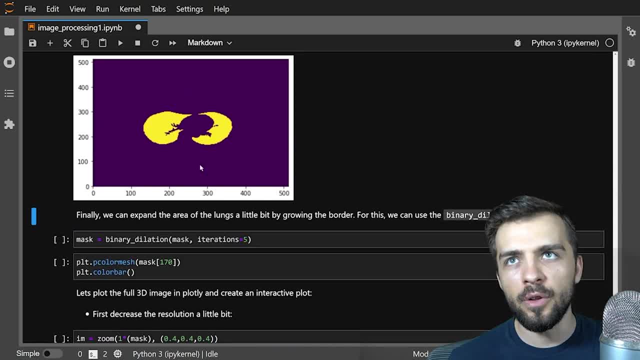 we have a 3d mask of the lungs. the final thing we can do is we can take these lungs, which are segmented- it's almost exactly where the air is. but we can grow them by growing the border a little bit, and for that we use the binary dilation function that takes an array of ones and zeros. 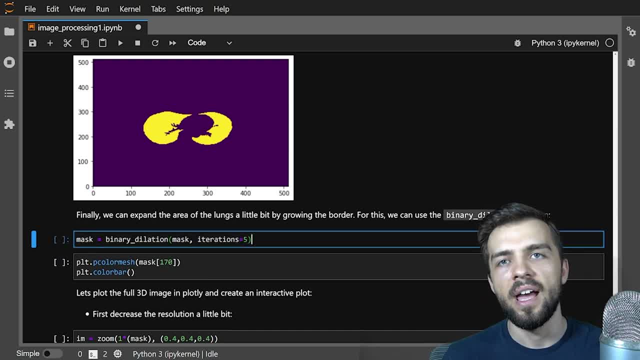 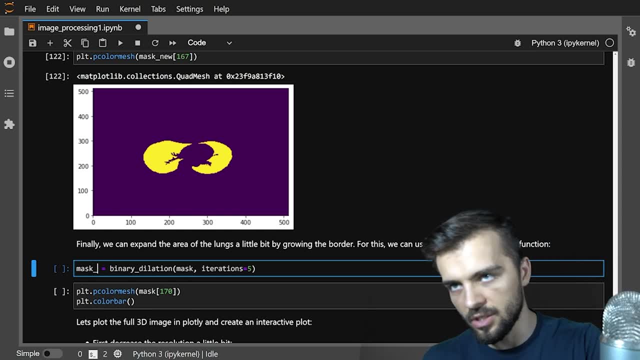 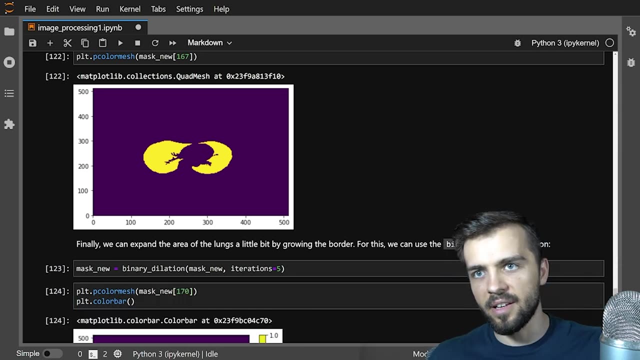 and it expands the border of the areas just a little bit and it depends on the number of iterations you use. so here i'm using five iterations. we'll use this on our mask new, so i'm gonna feed in mask new here and i can plot this and you can see that the area will be just a little bit more expanded so that. 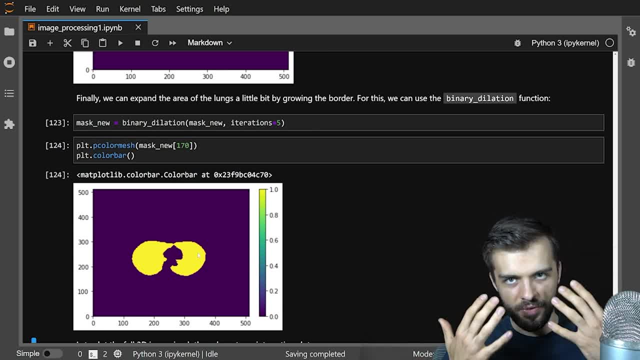 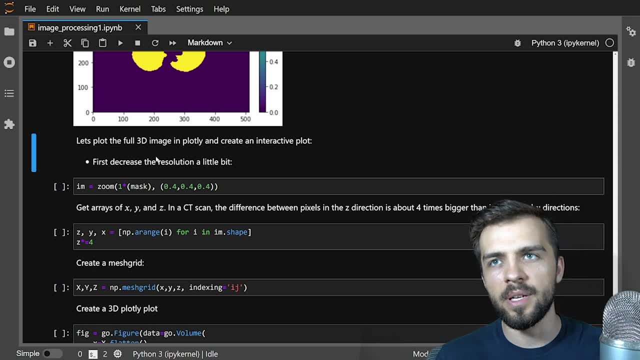 gives a little more leeway, so that your mask just sort of not only takes in the lungs, but it's a little bit bigger as well. so finally, we'll- we'll create a 3d image in plotly, and now this is a very resolute image. so what we're going to do is we're going to reduce the quality by about 40. 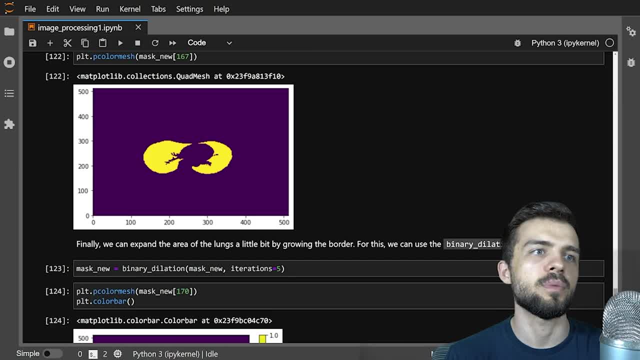 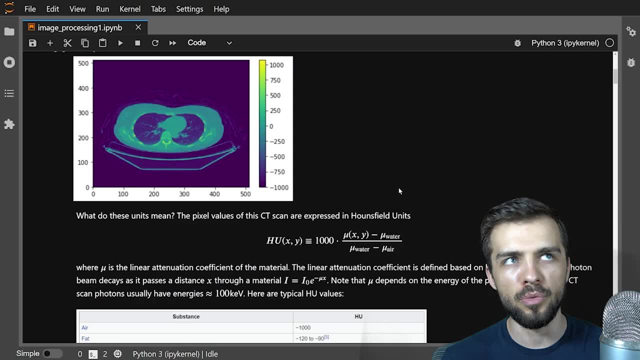 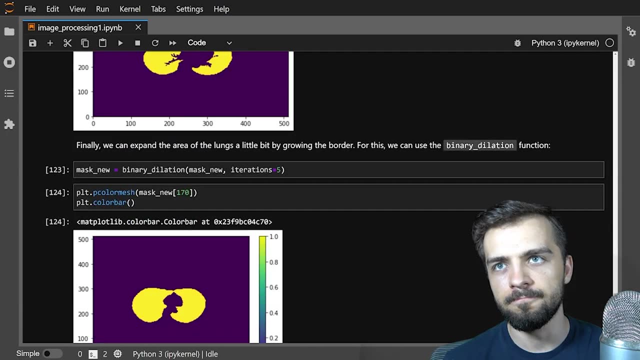 so that's what, also what i imported from the nd image library, uh, sorry, from the yeah, right here i ported the zoom function. what that will do is it will take an image and it will reduce the quality by 40, so that means that the resolution decreases. so instead of being 512, maybe it's 200, and 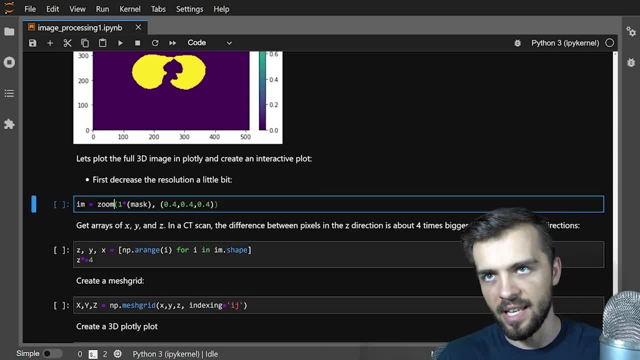 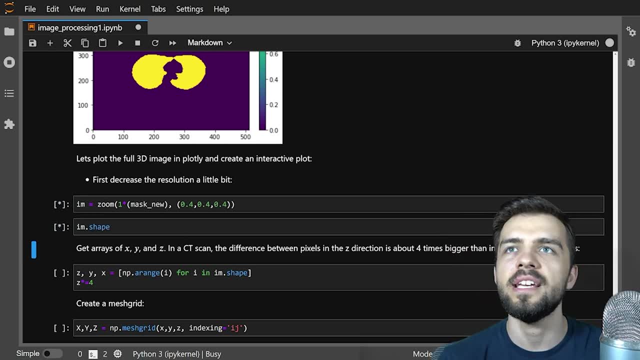 something, and so, uh, that's what i do and i get this image here. so now, if i look up the shape of my image, you'll see that it is no longer 512 by 512, but it's shrunken by 40. so it's the same sort of thing. 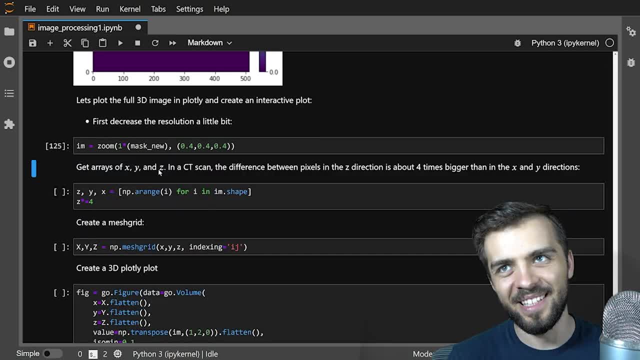 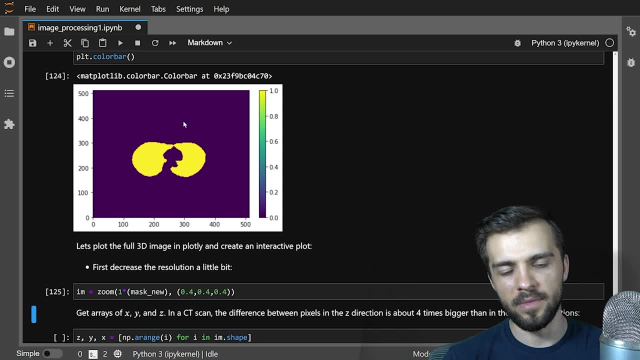 here you just lose resolution quality of the image. then we're going to get a raise of x, y and z. so in a ct scan, by the way, the x and y uh distance here, so in the 512 by 512, is about one-fourth the size. 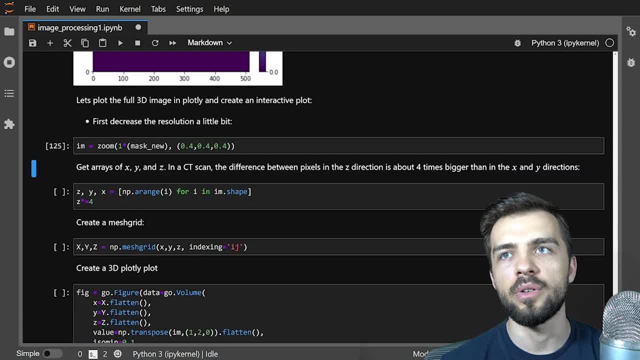 of the distance between separate z slices. so in order to manage that, i create a raise of x, y and z and i multiply z by 4.. so i'm going to create a raise of x, y and z and i multiply z by 4.. so i'm 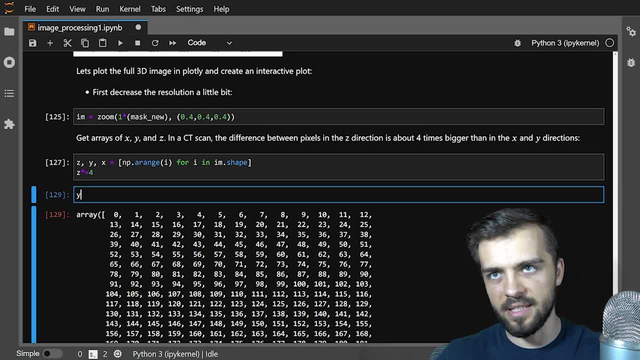 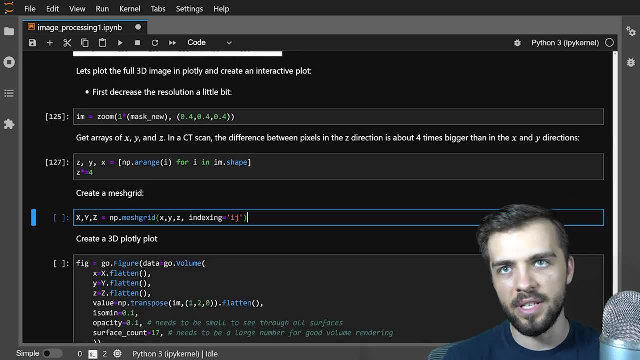 of the actual array. so the x goes like this, y goes like this, and z is in steps of four. this is going to be for plotting in plotly. uh, i can create a 3d mesh grid out of these three things. i'm going to have a video on this function. so then, what i do is i create a 3d plot in plotly. 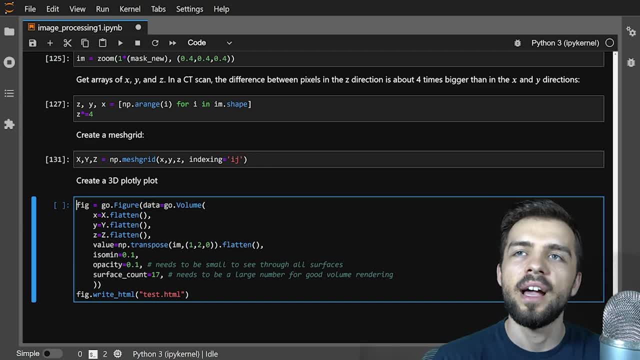 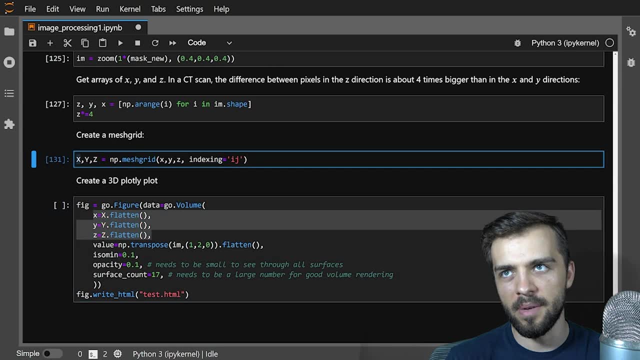 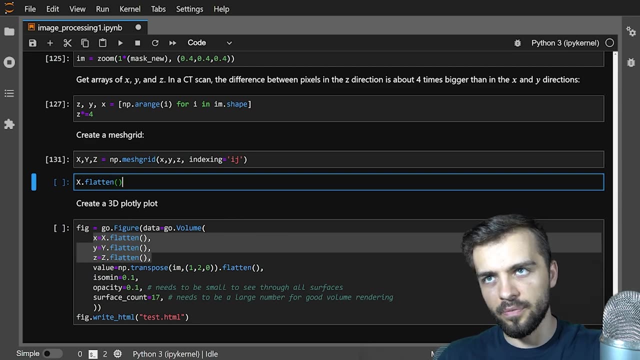 which i can then open in an html browser and so the data and this is going to be govolume. i feed in my mesh grid here and i make sure to flatten each of the mesh grids. so the mesh grid of, of course, is a 3D array. If I call flatten on it, it will sort of go like that. So this is what it. 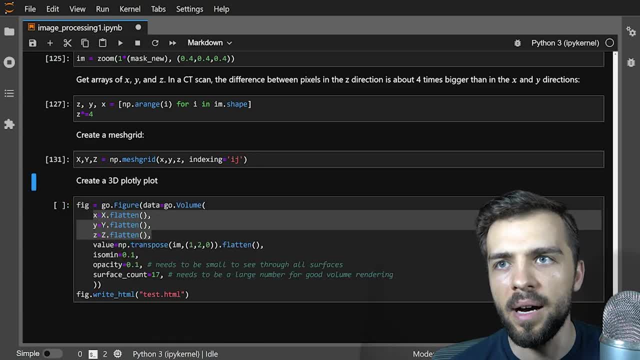 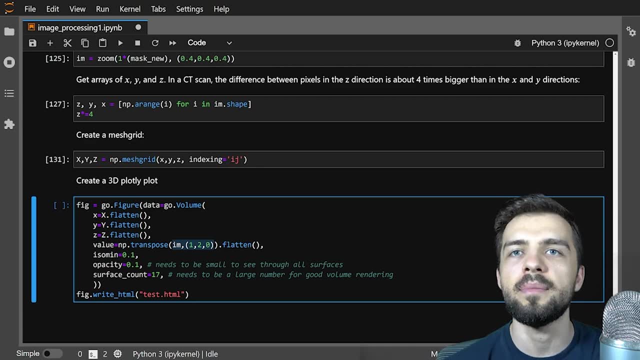 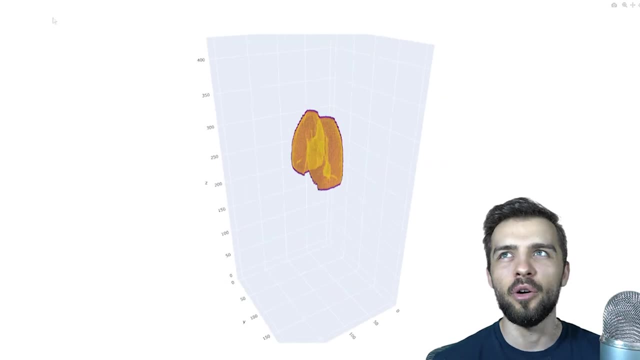 originally looks like. I also feed in my image here, making sure to transpose it a little bit so that it fits the right dimensions for the image. I make sure to flatten this as well. So all of these are 1D arrays and I can save it. And so here, by the way, I had to open the HTML file. 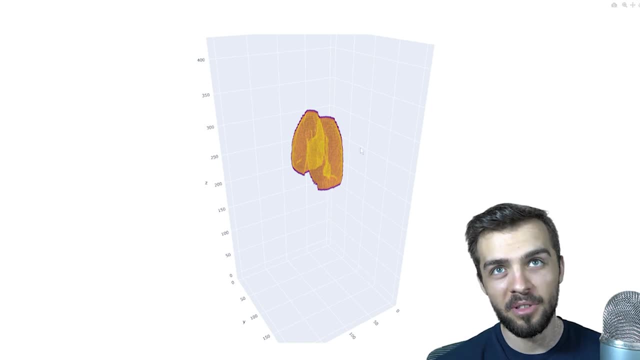 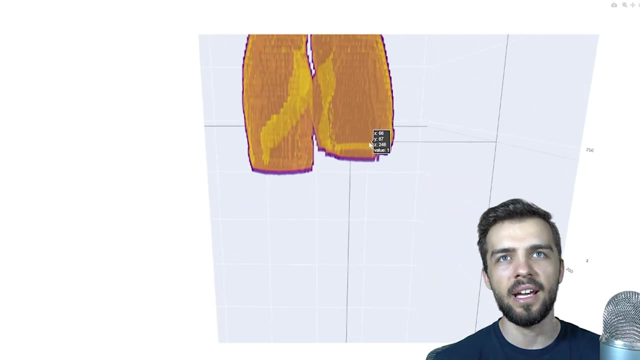 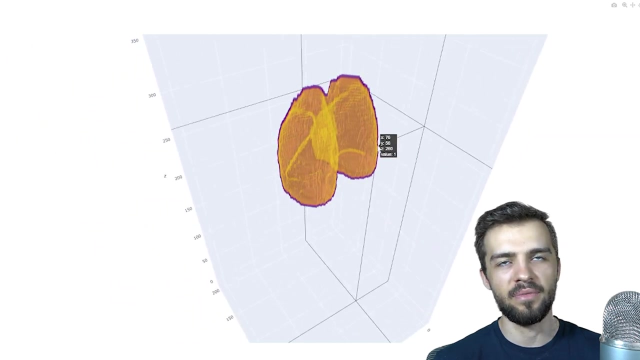 in Edge. It seems like Edge can do this better than Chrome, So points to Edge there. But I opened up this interactive HTML from Plotly And, as you can see, we have the two lungs segmented beautifully And of course the main purpose of this video wasn't quite the visualization at the. 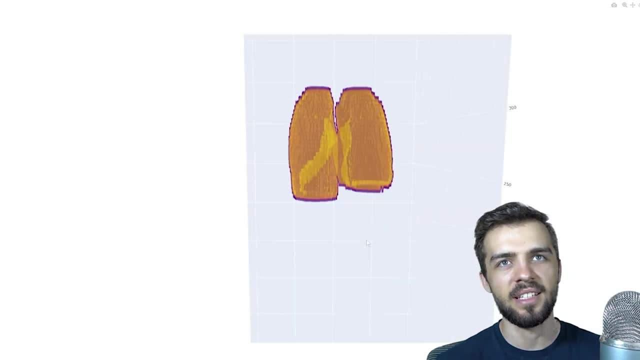 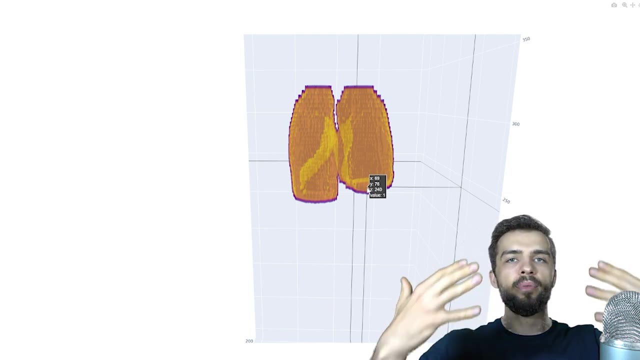 end. This is more just a tool for me to show you like all the slices at once, But the idea is that once you have a mask of a region of interest, it could be a lung, for example. in a scan it could be the heart. It could be any picture where maybe you have a car and you want to segment.